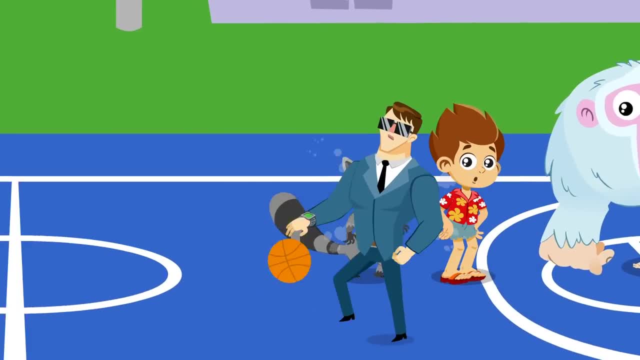 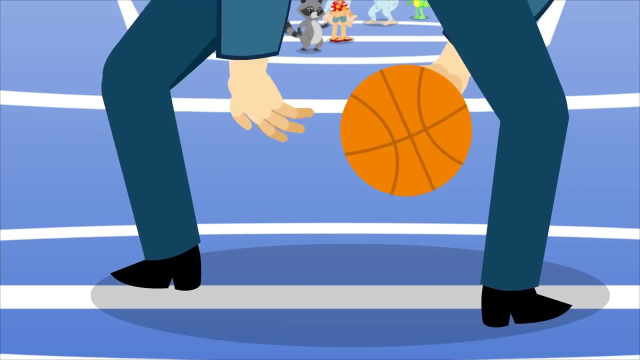 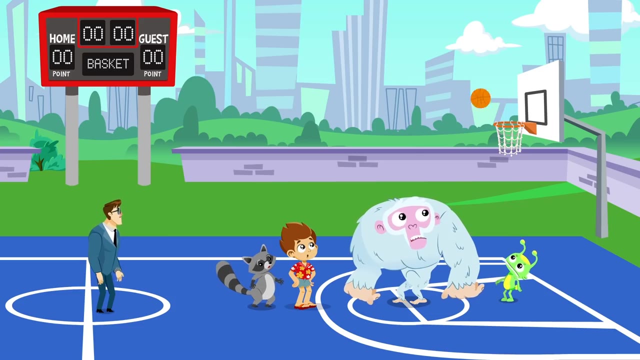 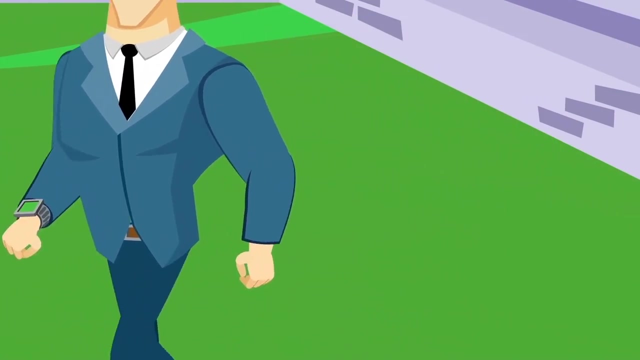 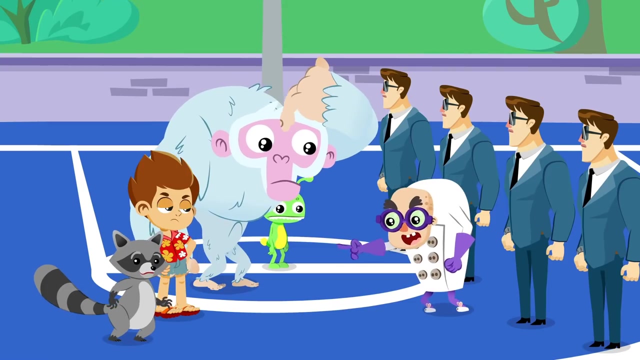 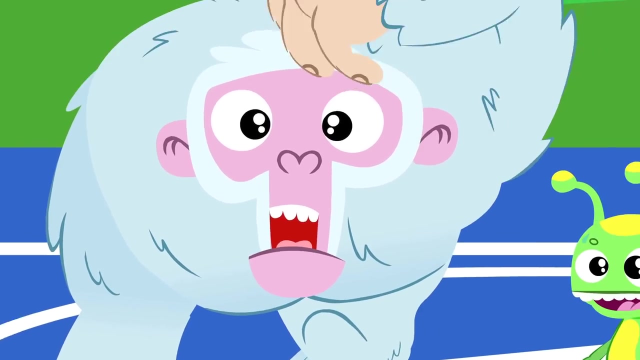 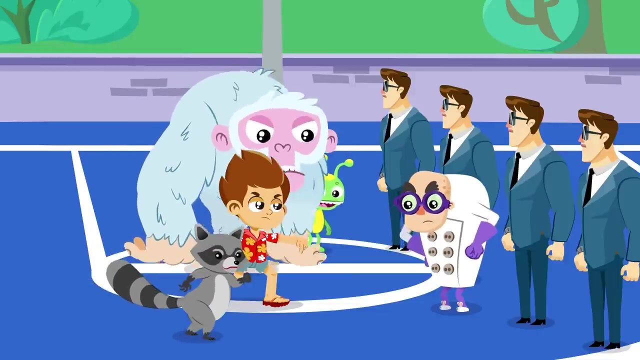 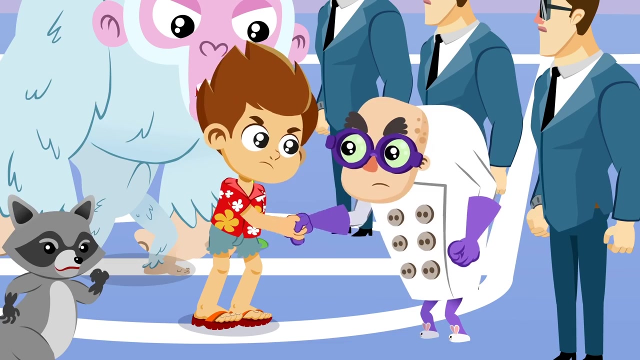 What They want to play. Yeah, I'm getting so dizzy. Oh no, What do you want? They want the court for themselves. That's not going to happen. The court is ours. Let's play a game and whoever wins gets the court. 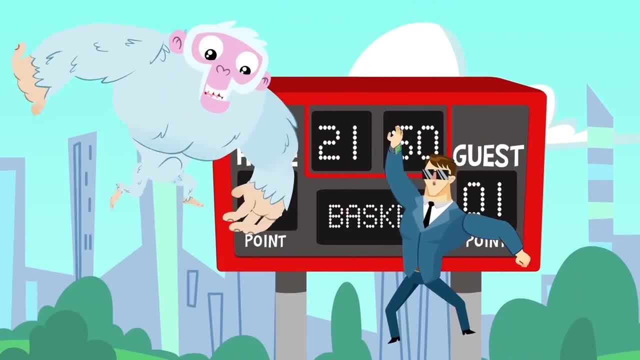 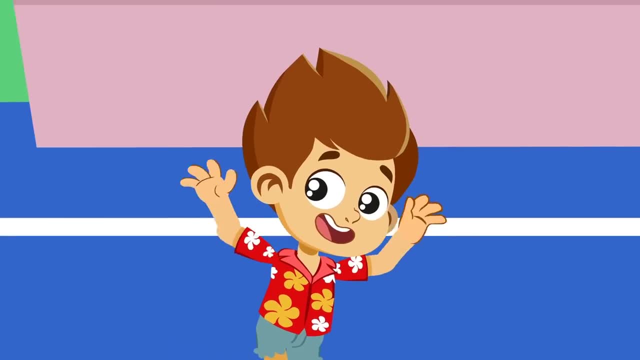 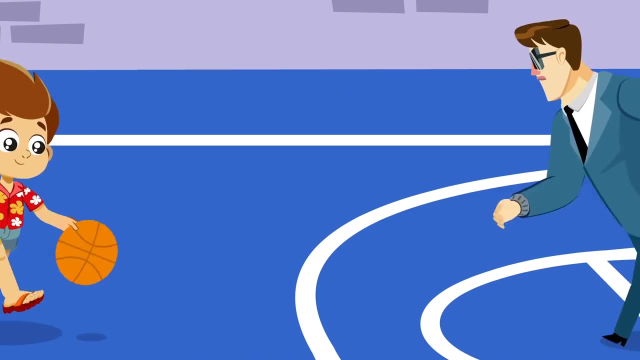 Ready, Let's play. Groovy takes the ball, but a minion tries to steal it from him. Ryder's open. Groovy passes, But wait, Another minion is getting close. Ryder bounces the ball between his legs and Raccoon dunks. 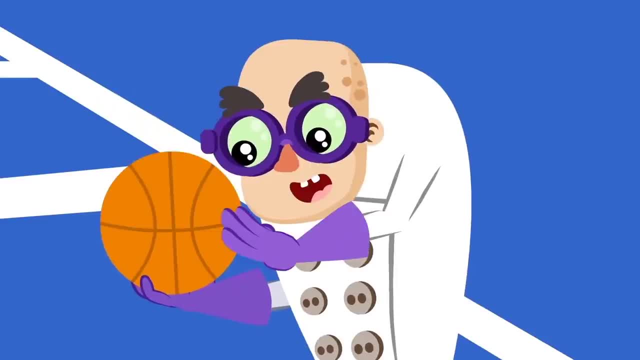 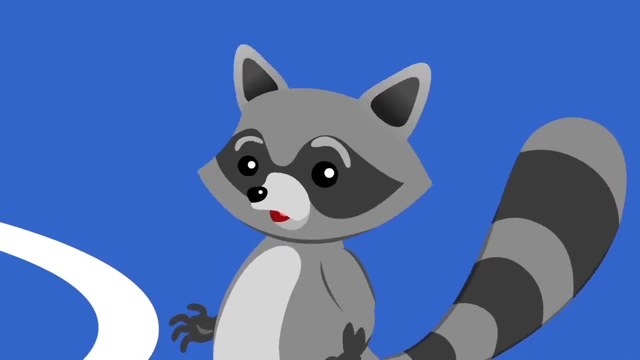 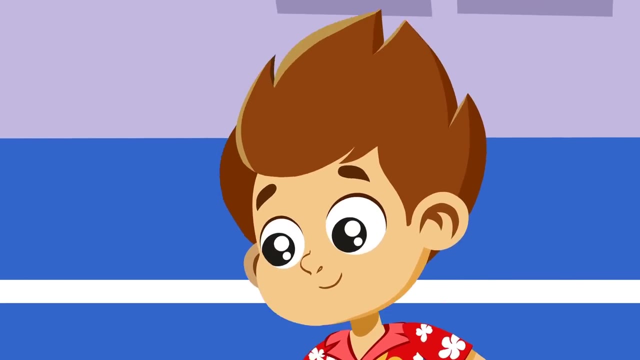 Hmm, what's Spooky up to? Is that a robotic ball? The minion sprints with the ball towards the basket. Raccoon tries to stop him, but Ryder stole the pass. Let's go, Ryder. Let's go, Ryder. 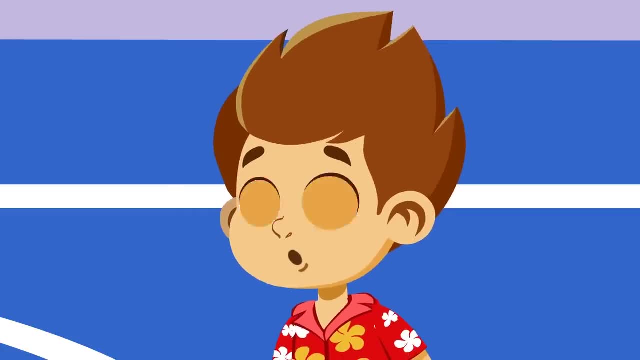 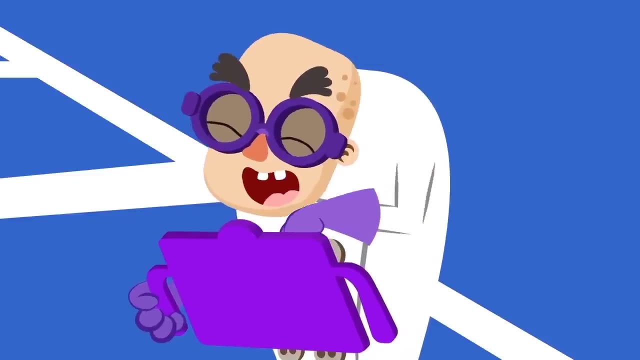 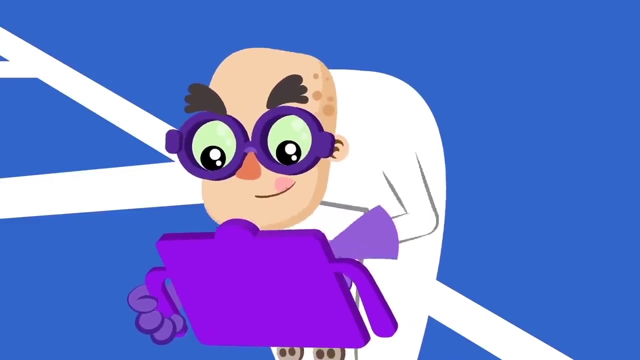 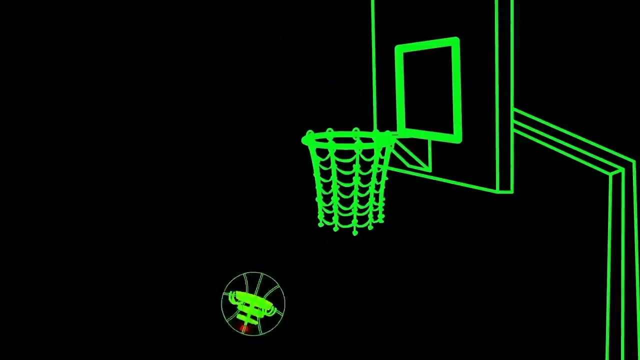 Ryder shoots and What Huh? The ball stopped in mid-air. It's Spooky. He's controlling it on his tablet. No, He moved it to the opposite basket And now he's scoring again and again. Kids, we have to do something. They're going to win. 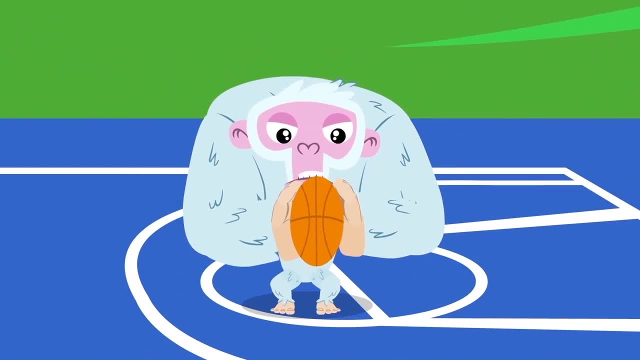 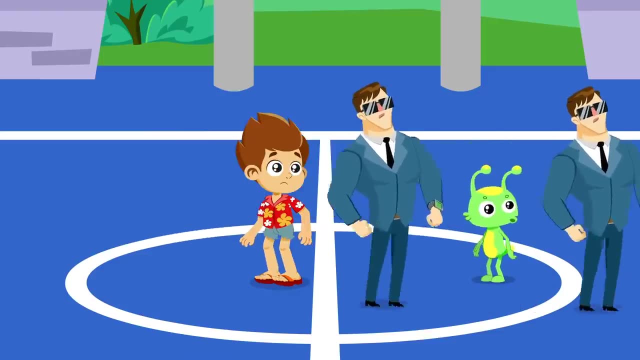 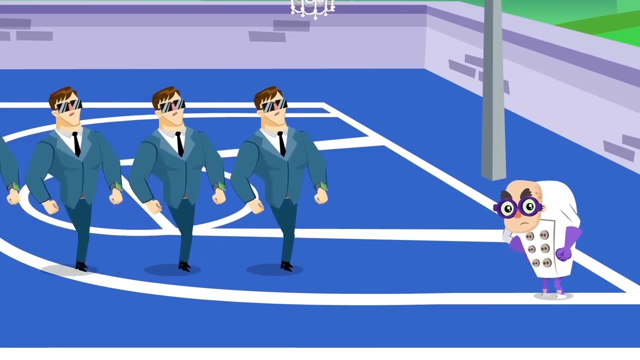 Monkey's got an idea. That's it. Monkey destroyed Dr Spooky's ball. Say goodbye to your evil plan, Dr Spooky, Or maybe, Uh-oh, He's calling his minions. What are you going to do with those tools? 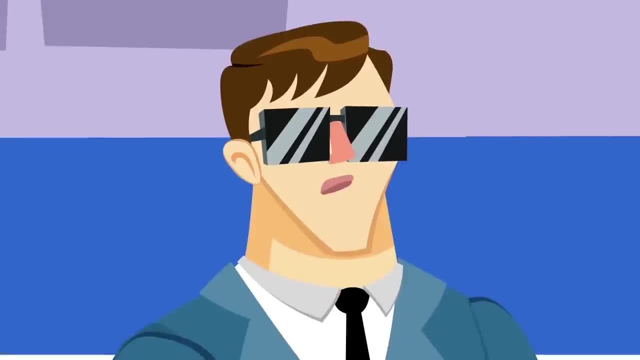 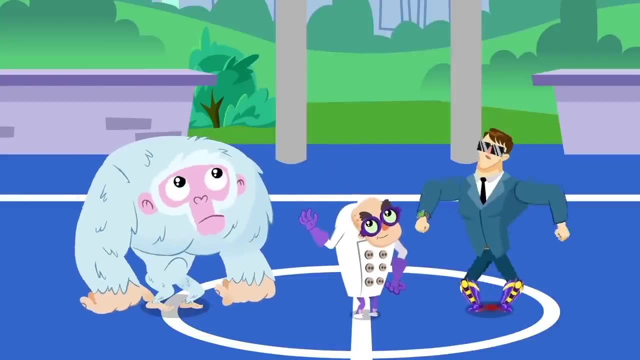 Some new shoes. I don't think that's going to be enough to beat our team. I don't think that's going to be enough to beat our team. Oh wow, The shoes have thrusters and now the minions can fly. 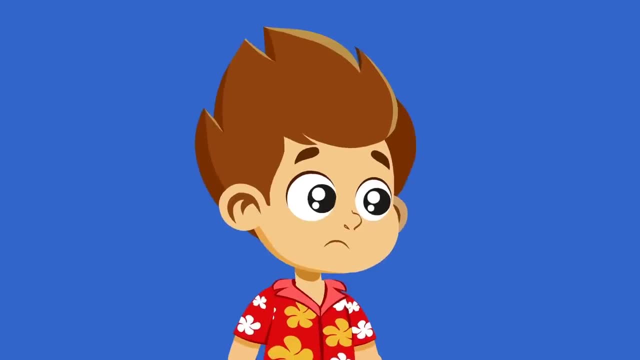 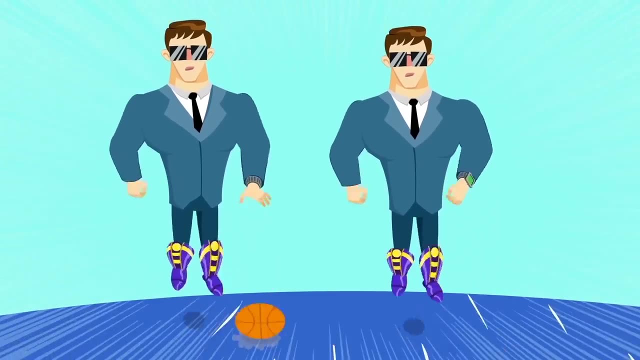 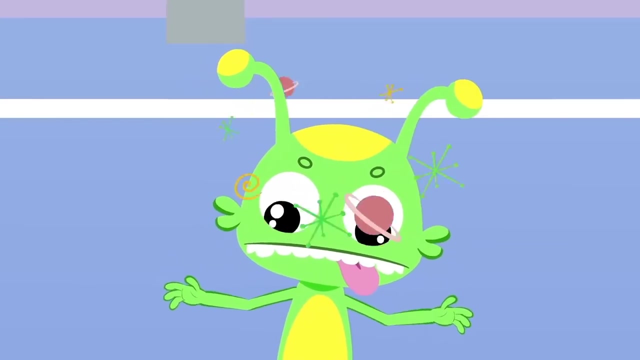 Go get him Raccoon Whoops. Maybe Ryder can stop them. Darn, it looks like he can't either. Let's go Groovy. We believe in you. Uh-oh Well, that wasn't your best play. 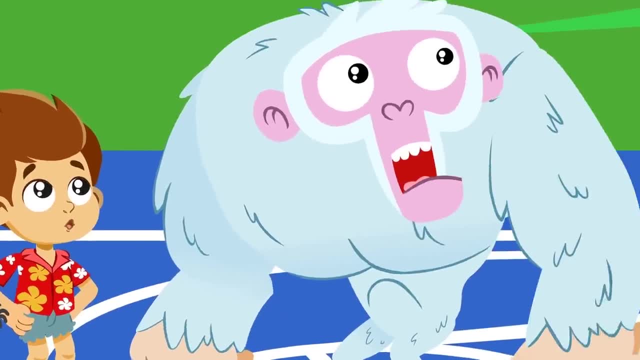 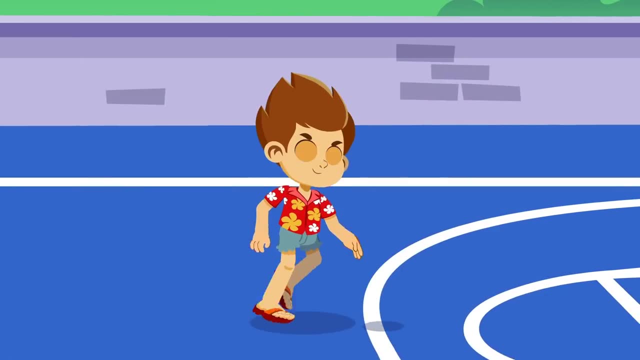 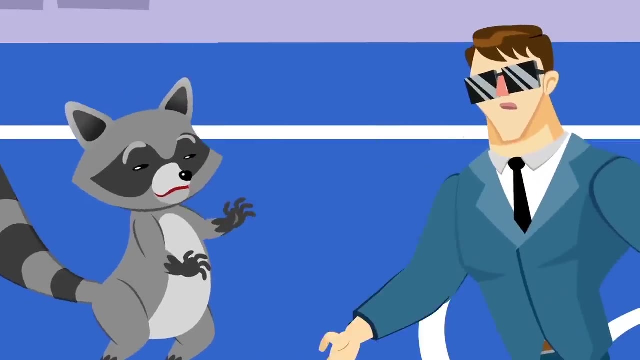 Oh no, Another point: It's going to be hard to make a comeback in this game, But you should never give up, Although sometimes maybe forfeiting in time is better. Sorry, but Dr Spooky's plan is definitely working well. 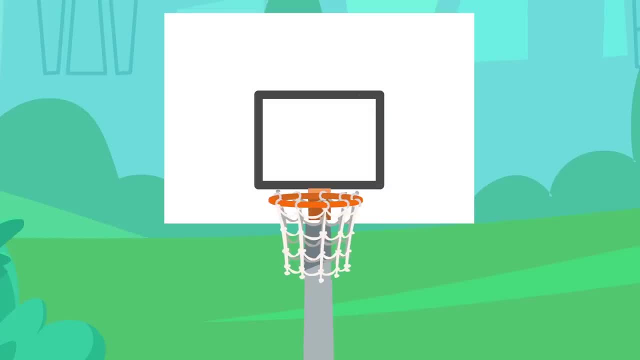 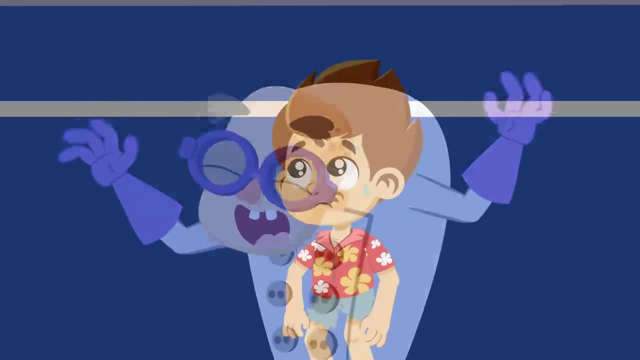 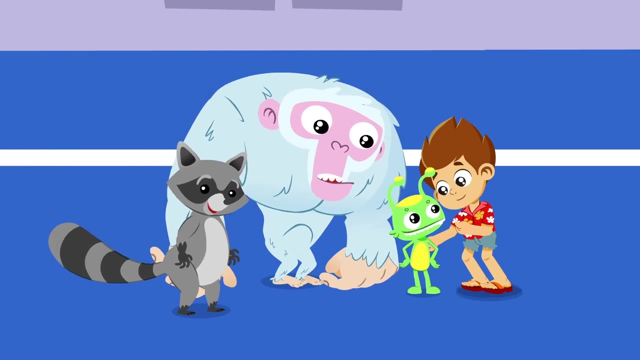 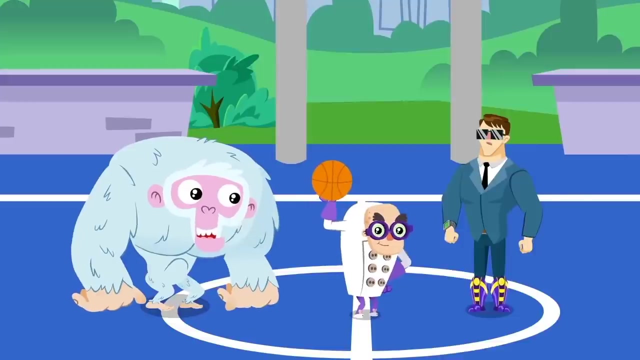 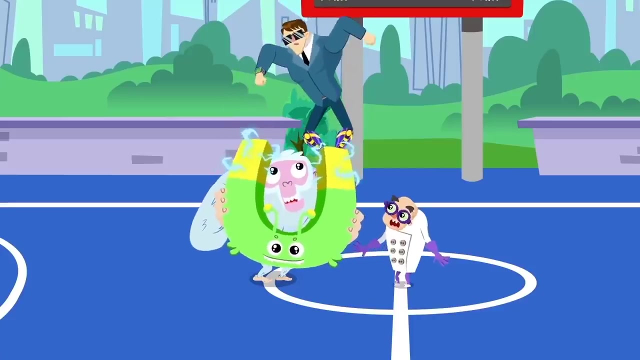 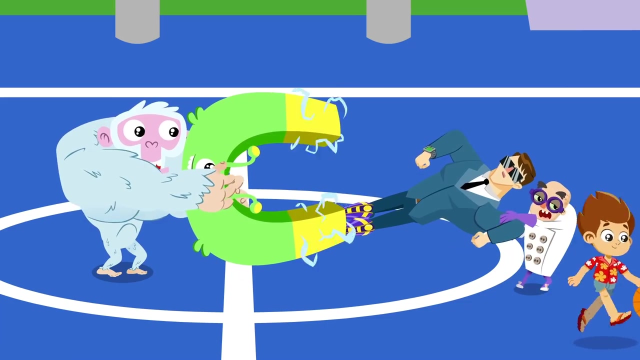 Too well, Let's go. Ryder Think: Groovy, Groovy, Groovy, Groovy turned himself into a magnet. What's your plan, kids? Oh, great Monkey is catching the minions with a magnet. Careful, Ryder, There are two minions behind you. 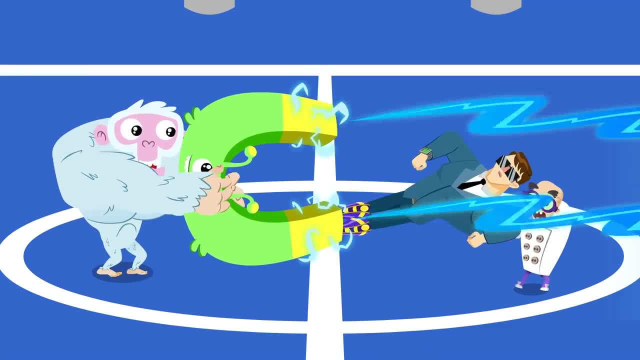 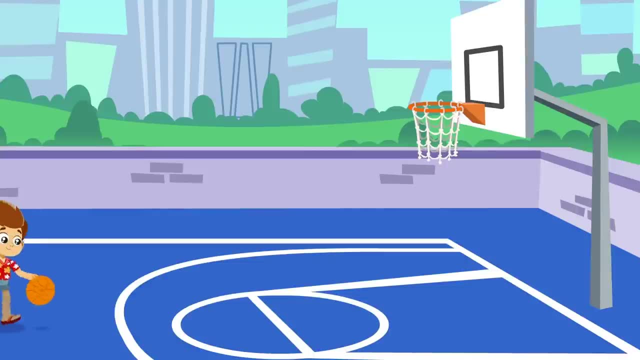 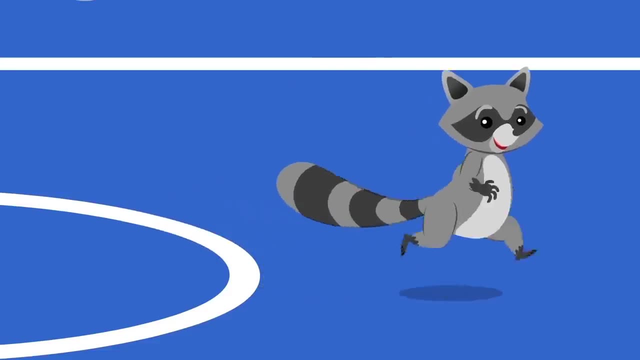 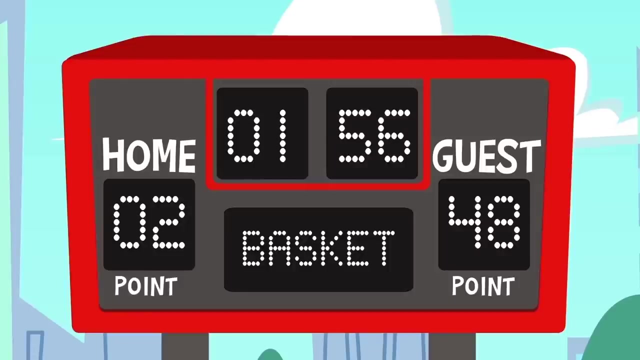 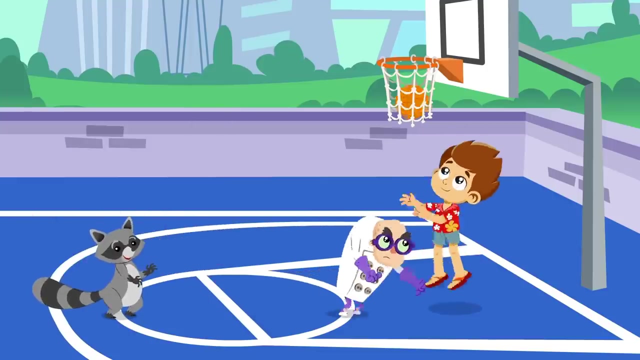 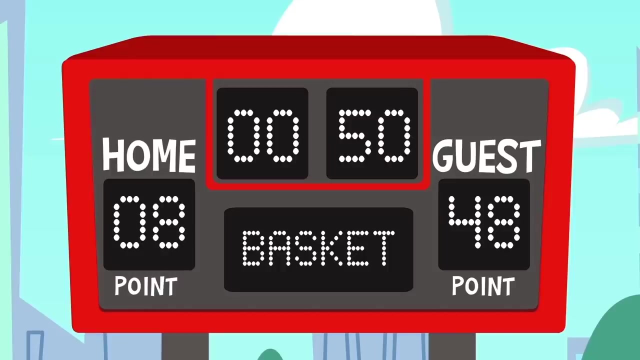 But Groovy and Monkey catch them And score. This is going to be easy. Groovy, Groovy, Groovy And Polar bear. Wow, There goes, Dr Spooky, Without your tricks you can't do anything. We can't stop this. 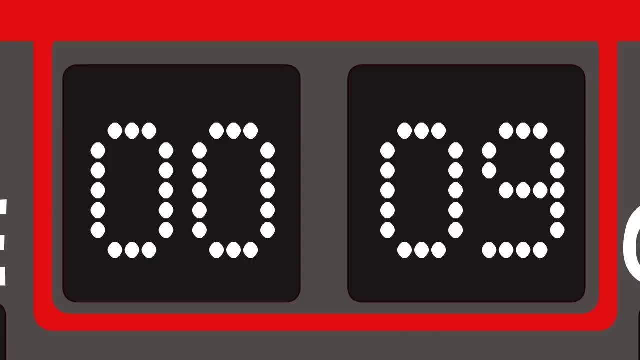 Spooky, you've got the key somewhere. you hotshot. What are you laughing about, Dr Spookie? Great, There's only ten seconds left in the game And there's a big difference in points. We've got all four points on your clock. 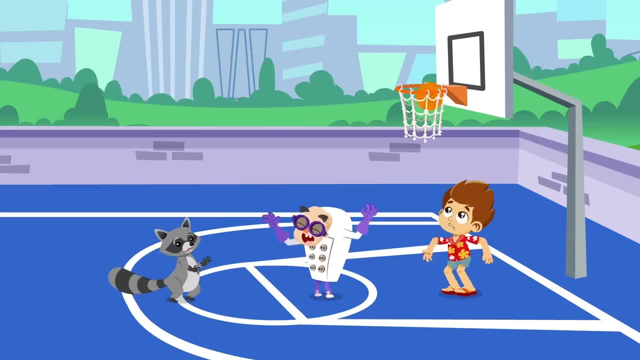 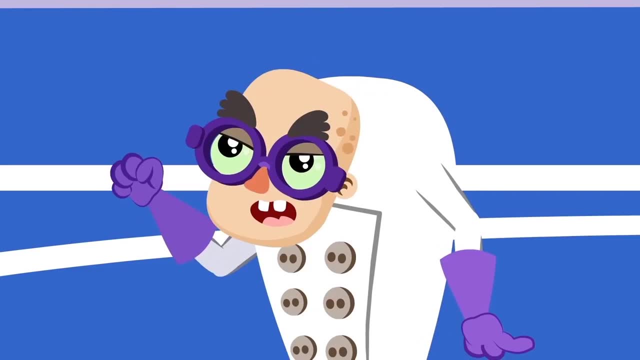 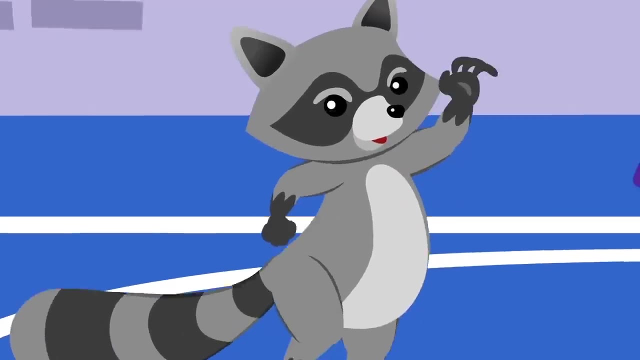 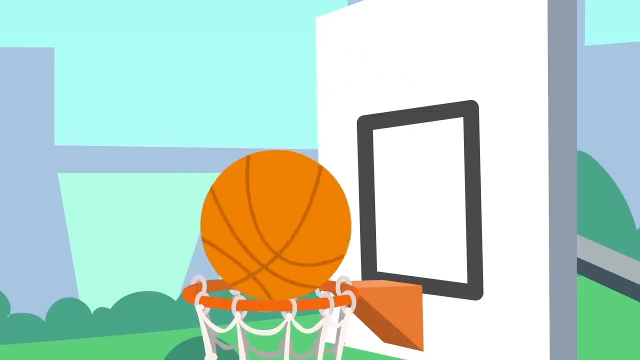 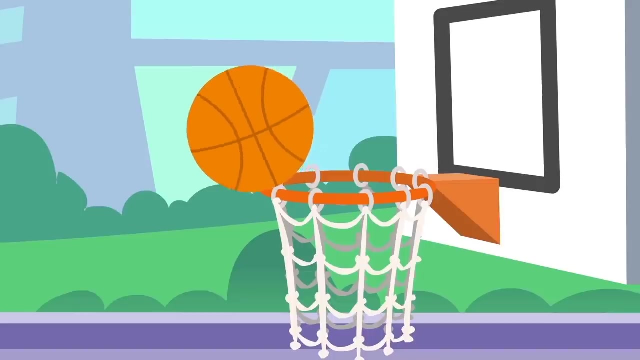 Hurry. Come on, kids, you can do it. There's only a one point difference. Darn you, Dr Spooky. Let's go, raccoons, Come on, go in, go in. Noooo, Wait a minute. the ball is going up again. 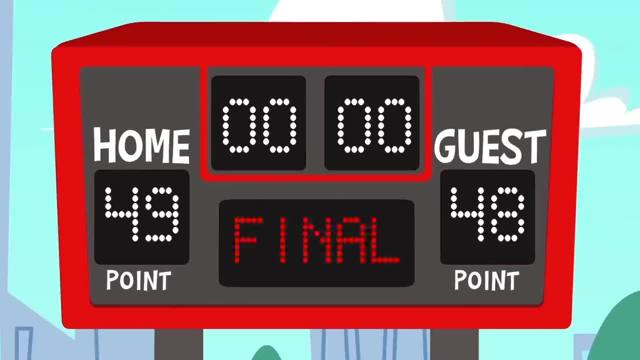 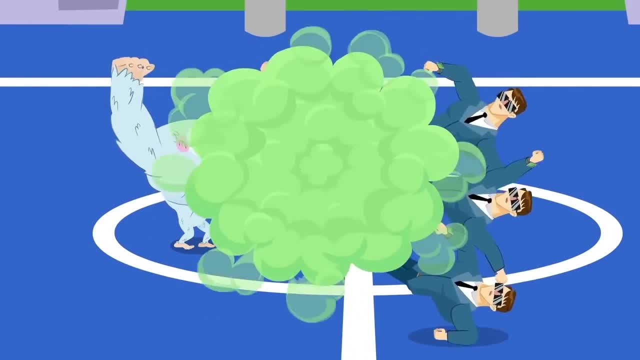 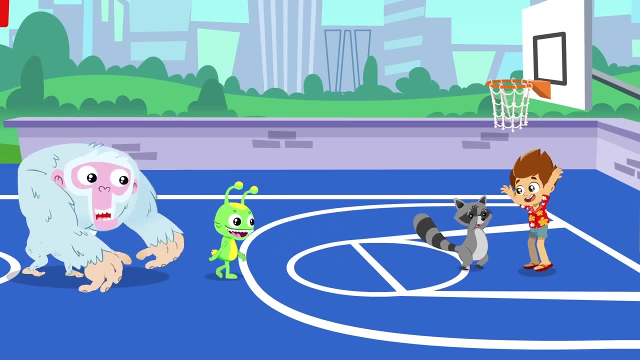 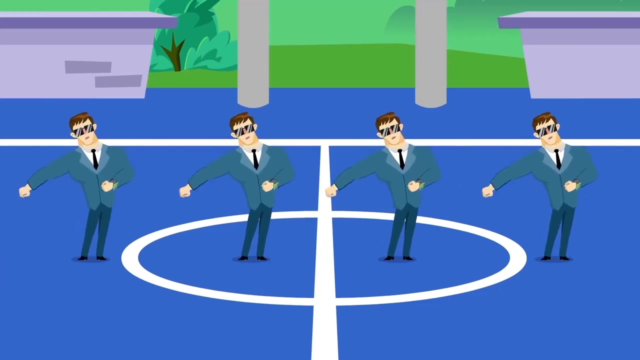 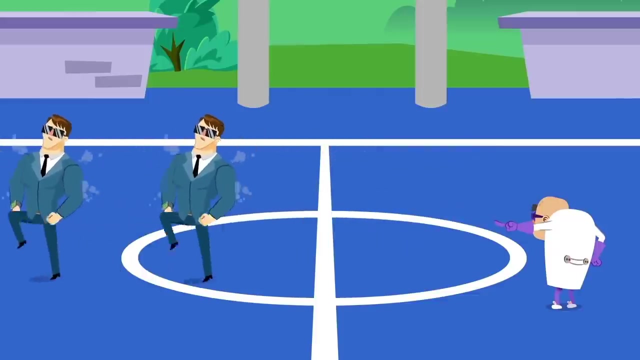 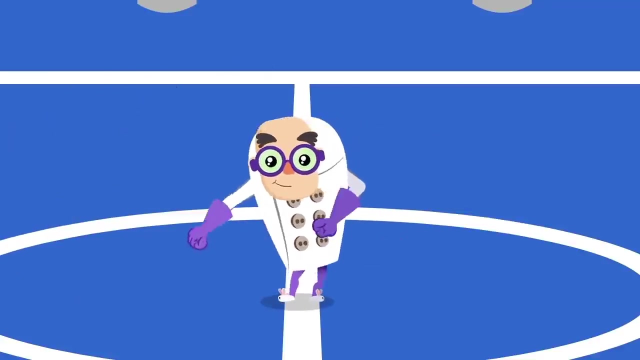 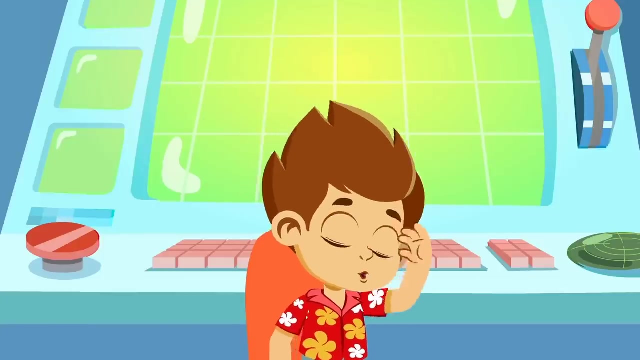 Ryder dunks at the very last moment. Bravo, You won the game. You're the best. Yeah, And even Dr Spooky knows you guys make a great team. Welcome to Kids Learning Corner. Today, we're going to learn about a new idea on how to save water. 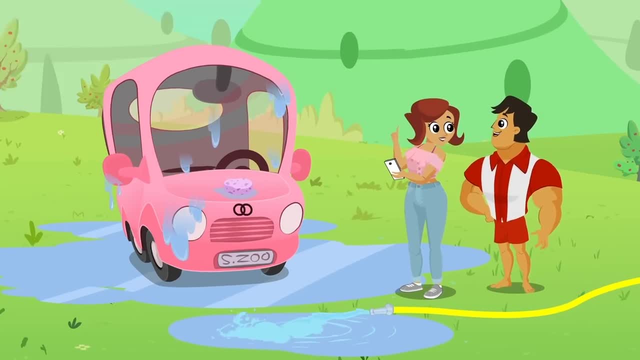 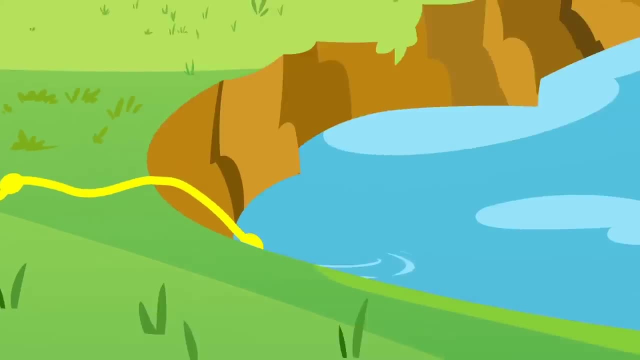 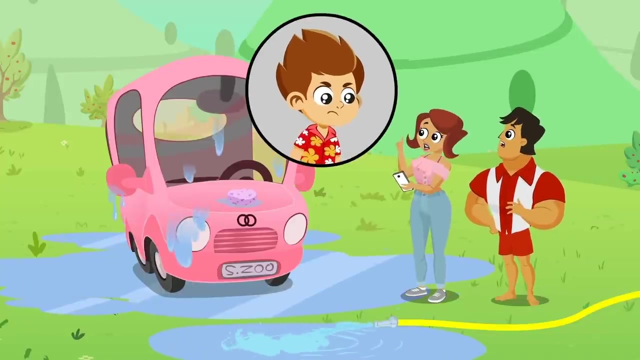 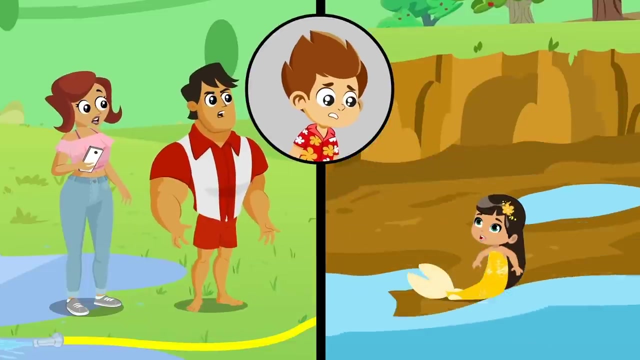 While your parents are washing their car. water is being used continuously, A lot of times unnecessarily. Hey, stop wasting water. Using so much of it hurts the ecosystem a lot. Look what's happening to the lake. The creatures that live in that habitat also feel the consequences of wasting water. 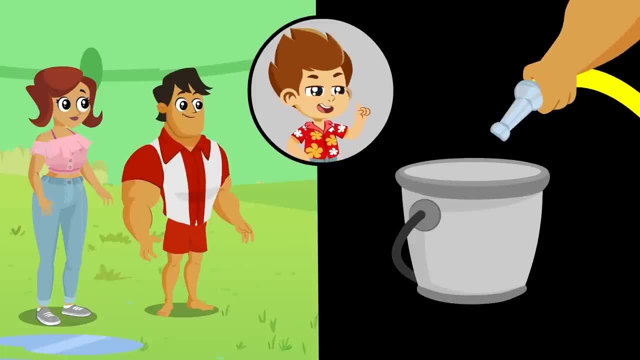 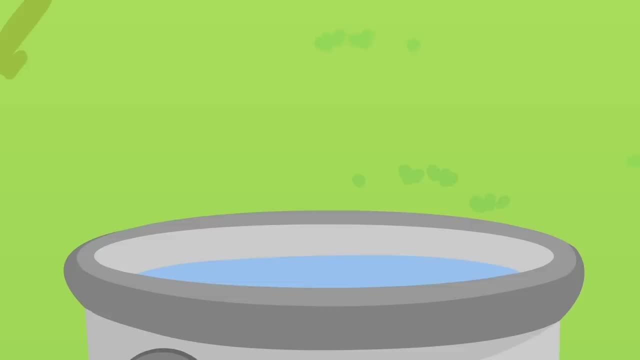 But like always, there's an ecological way to do things Right, Kit. If we fill up a bucket, we won't need to have the hose running while we wash the car And we won't waste any water that way. Get to work, Mom and Dad. 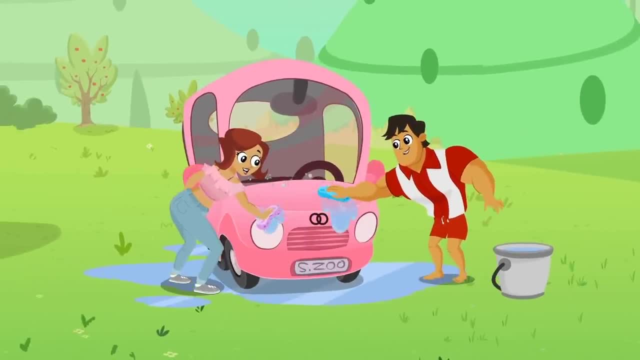 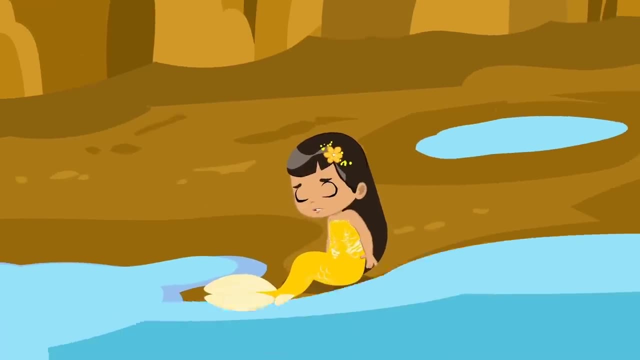 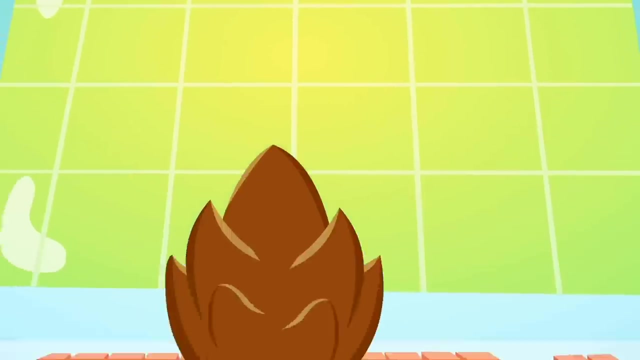 You see, it's a very simple gesture that can make the planet a much more sustainable place. We can save the environment together. Great Remind your parents to do this next time you're with them to wash the car. Let's save the environment together. 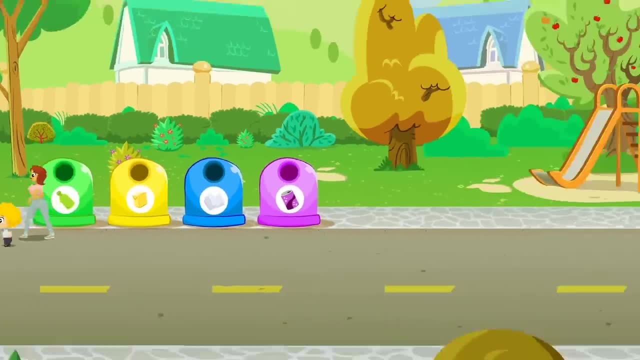 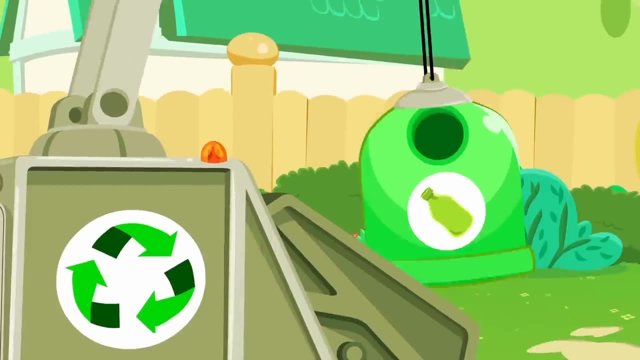 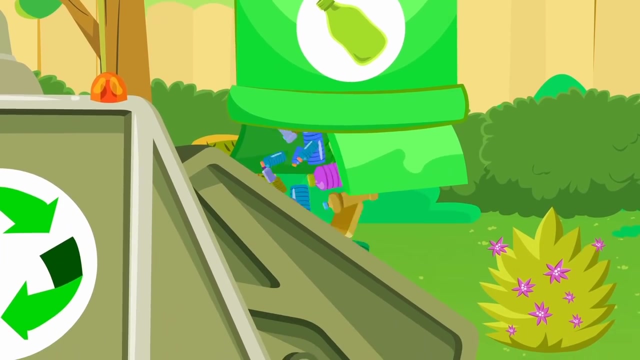 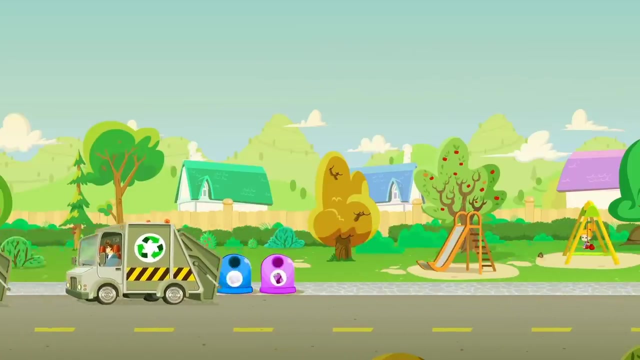 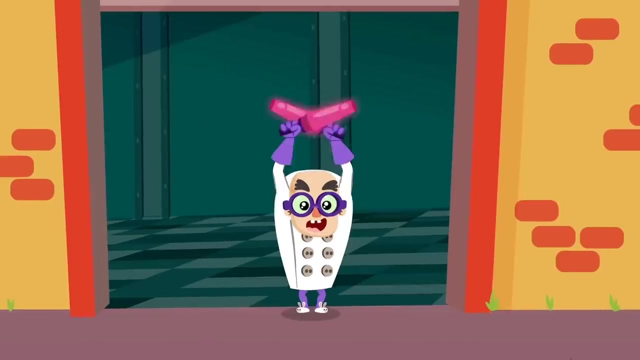 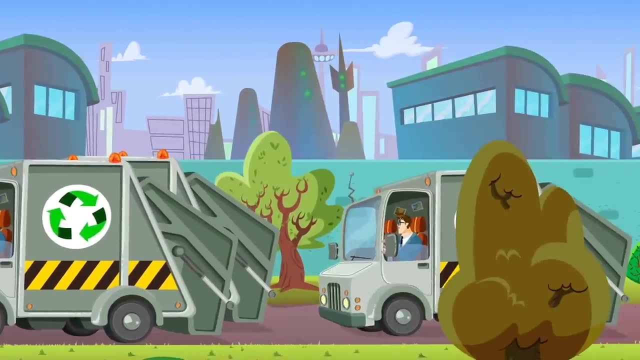 Just what I like to see: Recycling to save the planet, Super zoo style. Hmm, Um, do those drivers look weird to you? They seem familiar somehow too, To the recycling plant. What Dr Spooky? Of course The drivers are spookers. 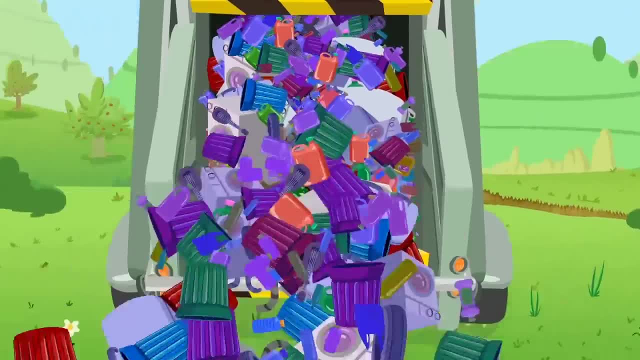 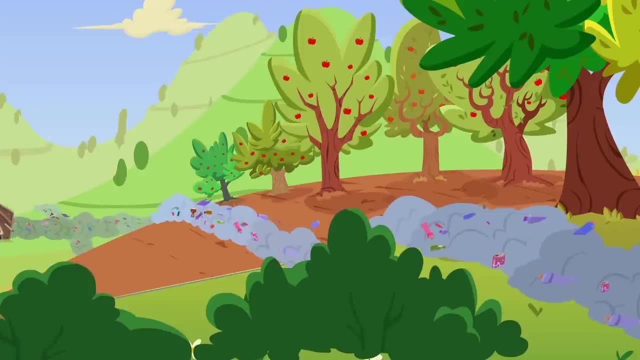 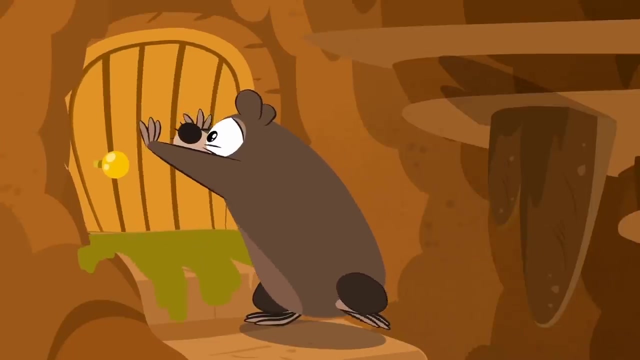 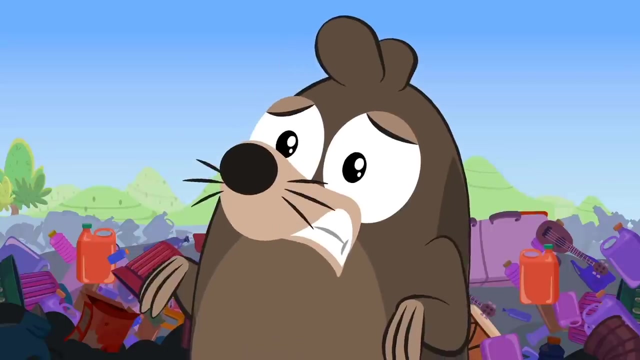 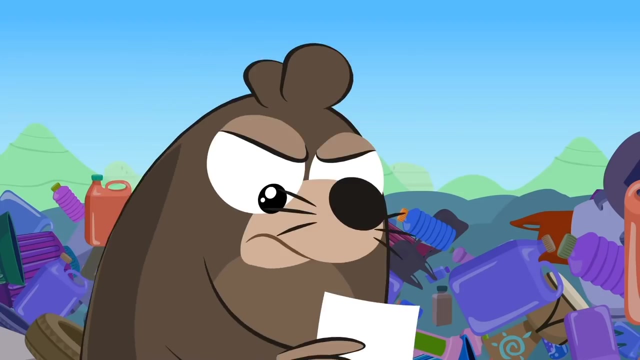 Where is Dr Spooky sending them? No, They're getting trash everywhere. Stop Please, Mr Mole. look how Dr Spooky and his henchmen have left everything There. those hooligans are. We need to get help. 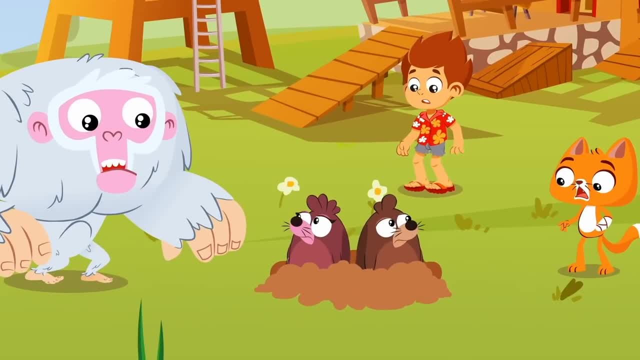 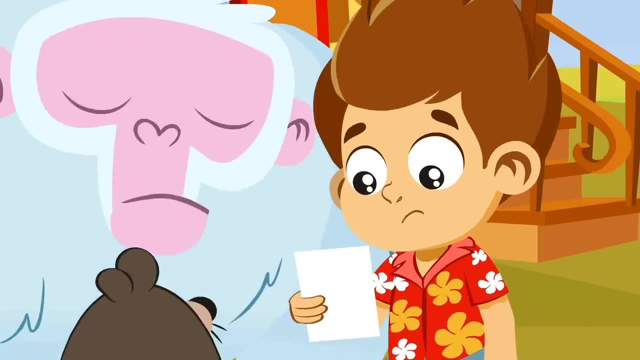 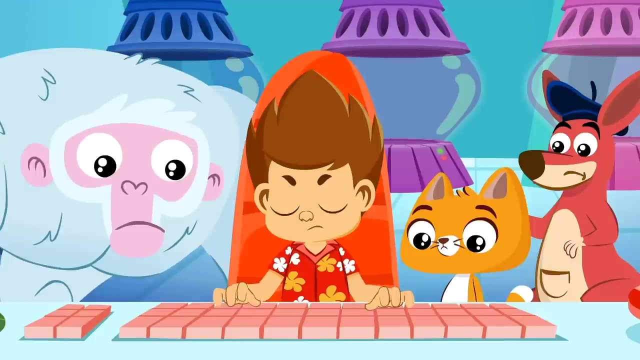 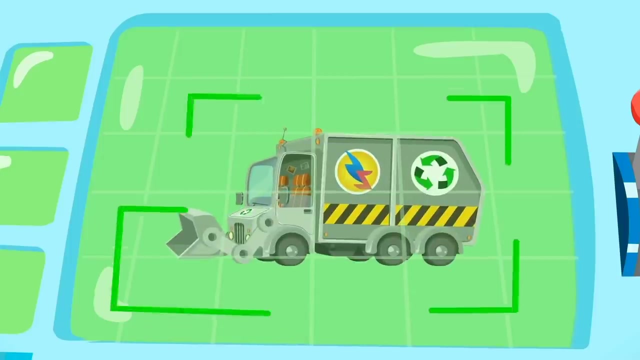 And here are the best superheroes in the world: Kids, Kids, Focus. Look, Dr Spooky has done it again. Kit, Show us the solution on your computer. Aha, We have to collect the trash and get it to the recycling center. 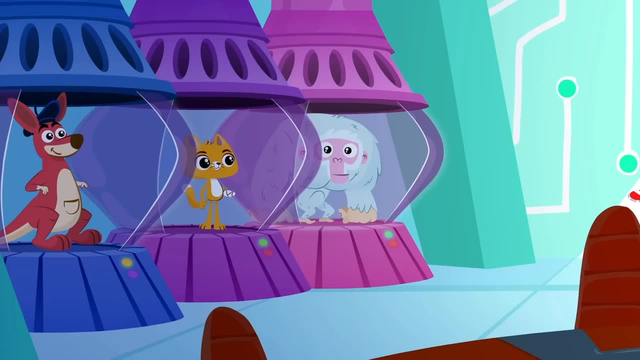 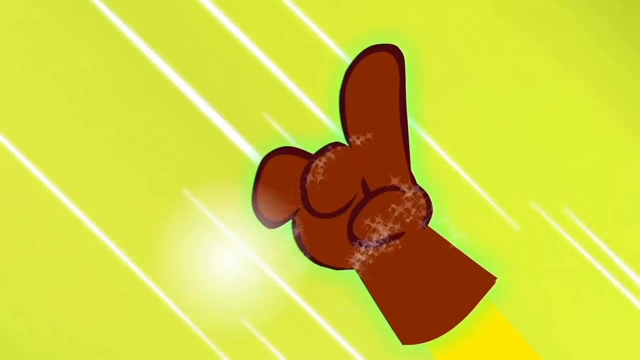 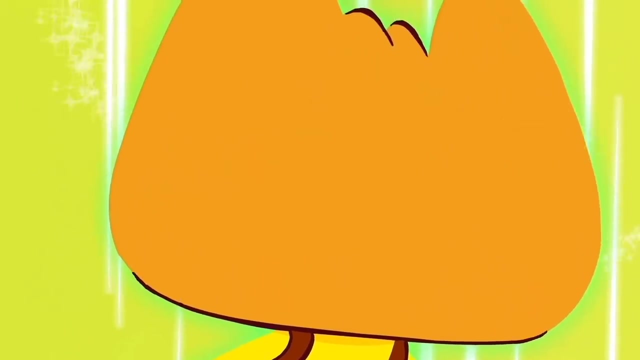 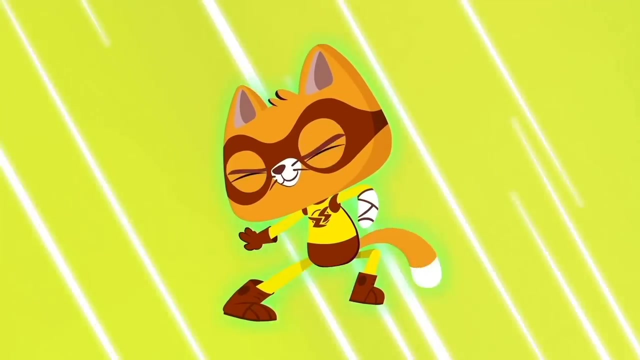 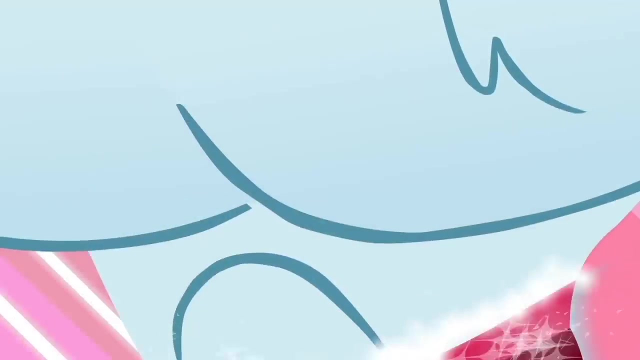 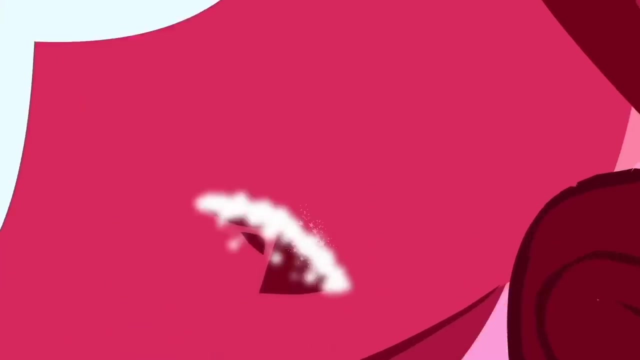 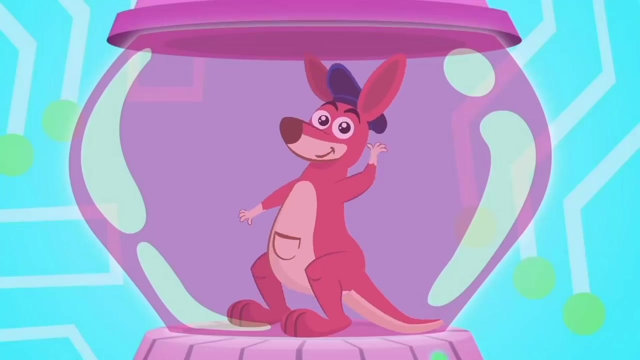 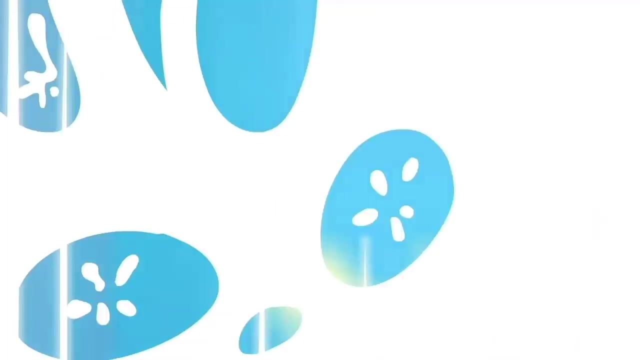 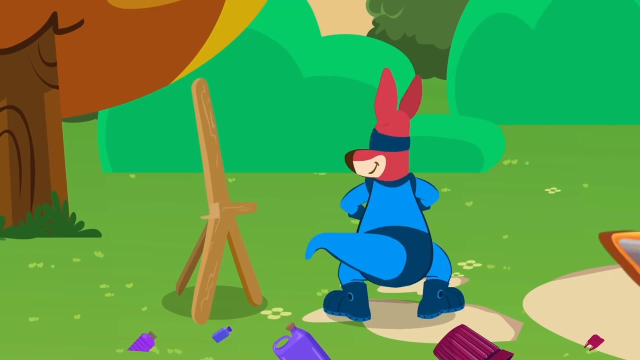 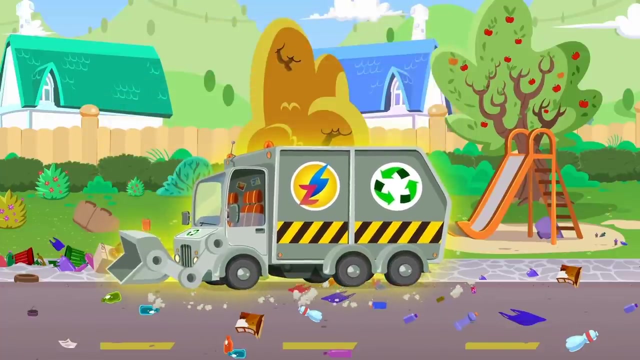 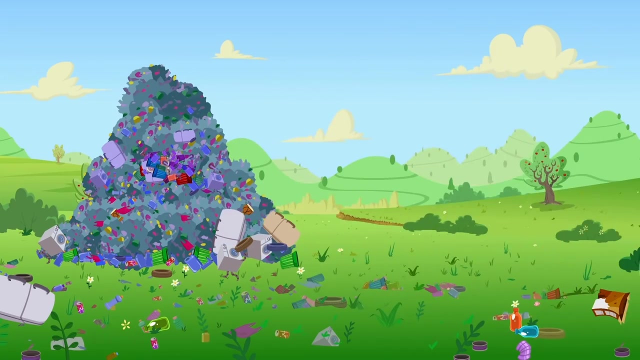 To the transformation capsules. The Caddy, Oh Ho, Ho, Ho, Ho Ho, Monkey, Kangoo, We're going to save the planet. Paint us a huge trash-collecting truck. Kangoo, We're over here, knuckleheads, Come and get us. 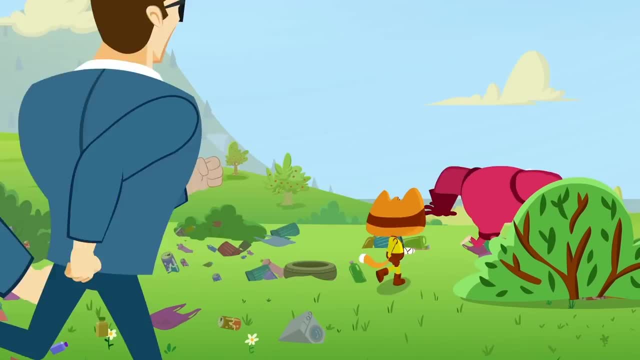 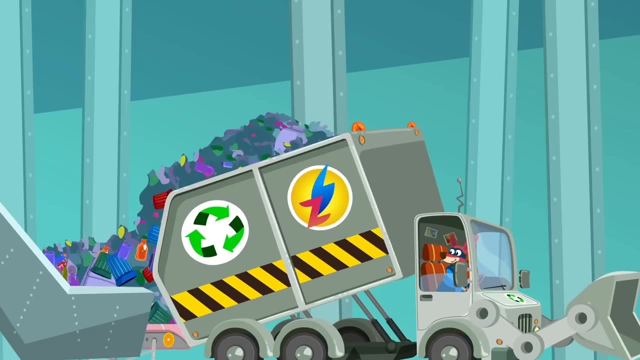 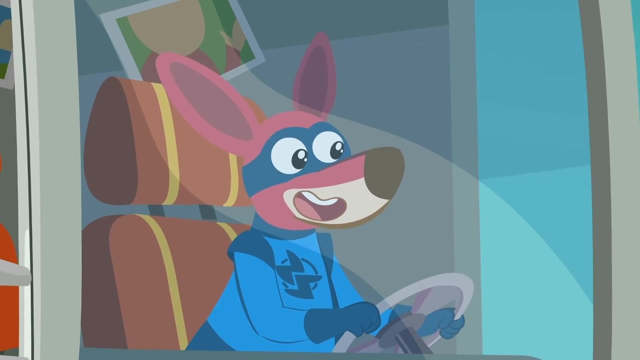 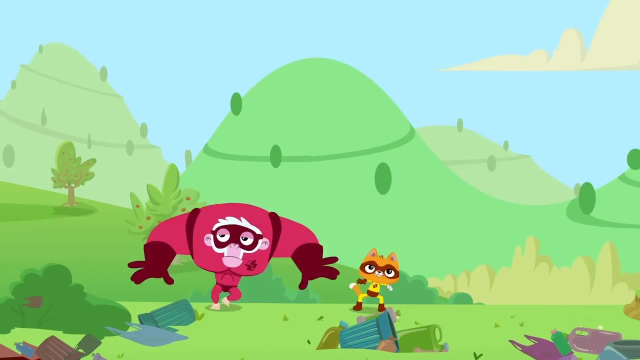 And in the meantime, Kangoo will collect all the trash. That's it, Kangoo. What It's great to recycle. Oh no, Dr Spooky summoned his robot, Monkey Catty. We have to help Kangoo. 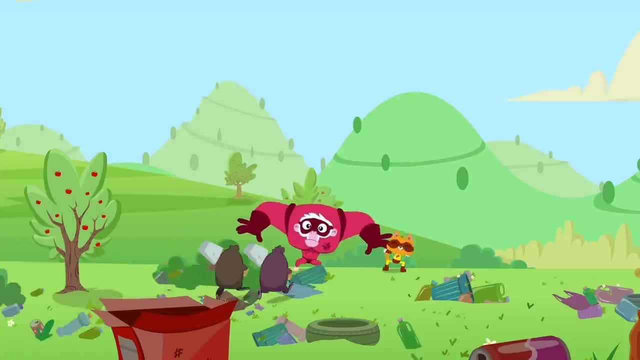 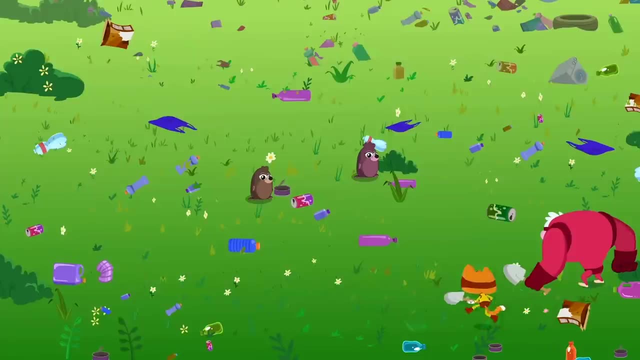 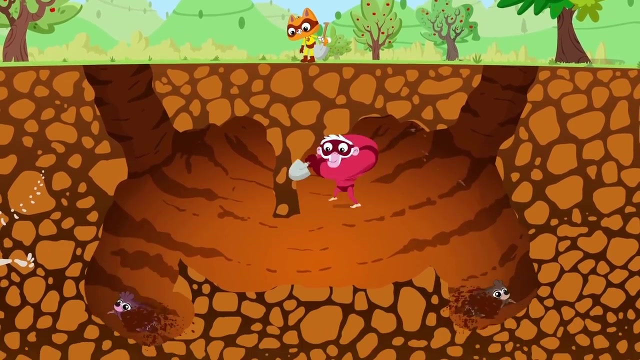 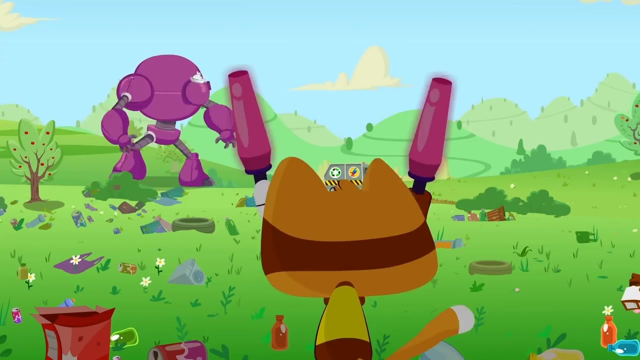 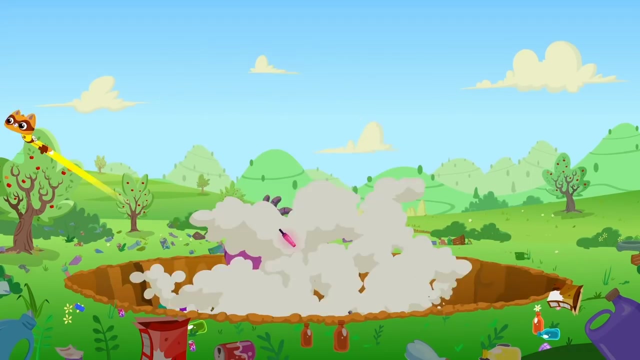 Aha, We have some new allies. We have to think of an emergency plan. That's some trap you're setting Great, And that's where you'll stay. losers. Little robot Come over this way Just where we wanted you. 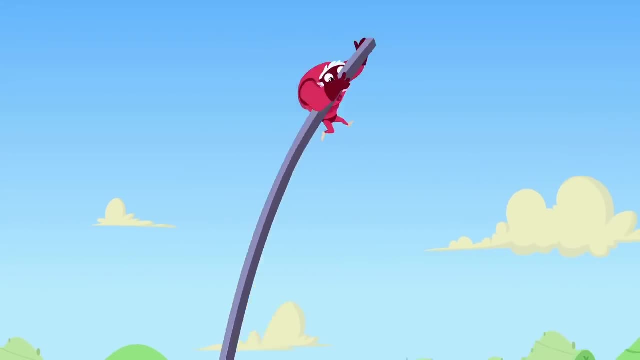 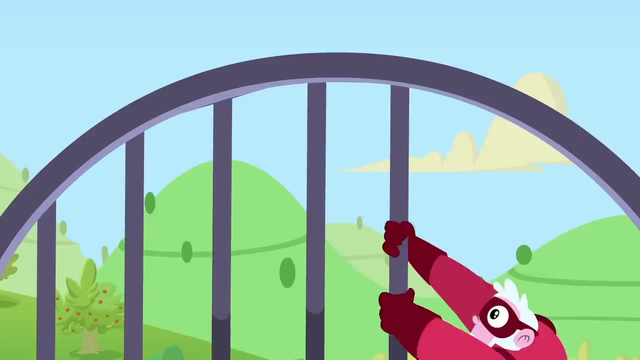 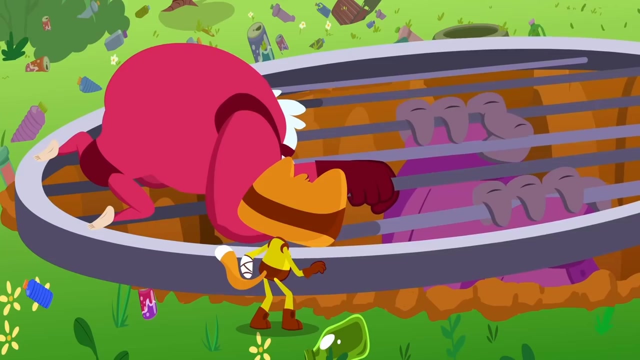 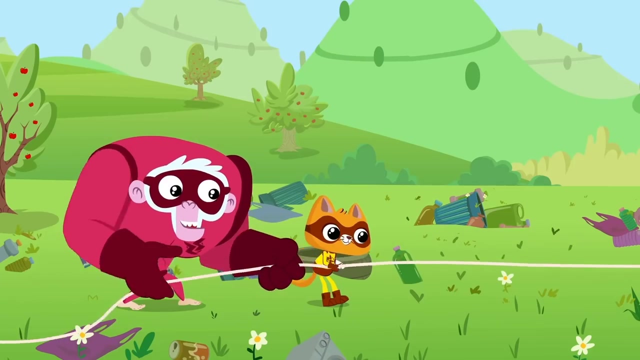 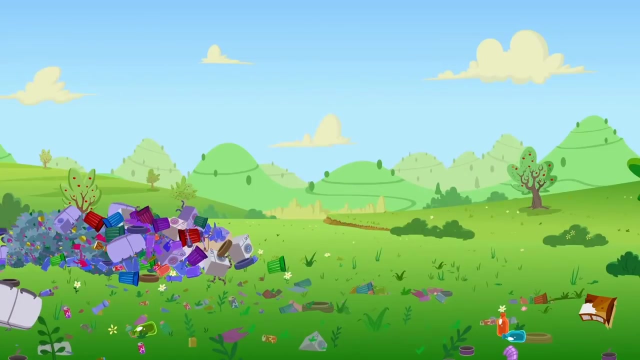 What is Monkey doing? Oh, a super-resistant grate. Now, that's a great way to recycle, And we still have to deal with you guys. Haha, Look at the bunch of knuckleheads that Catty caught. Look how clean everything's getting. 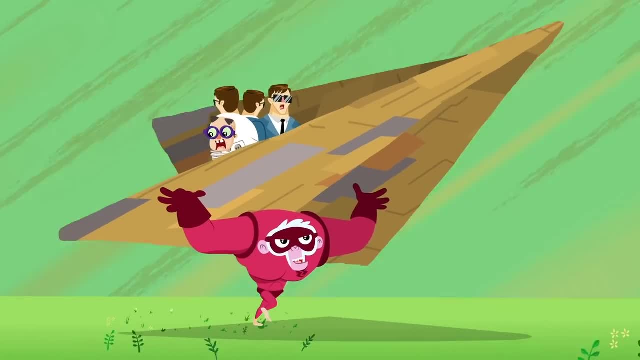 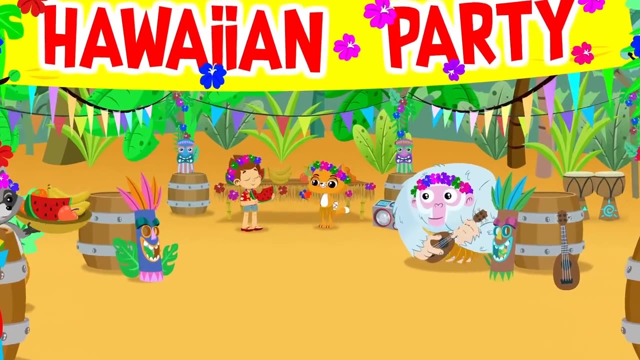 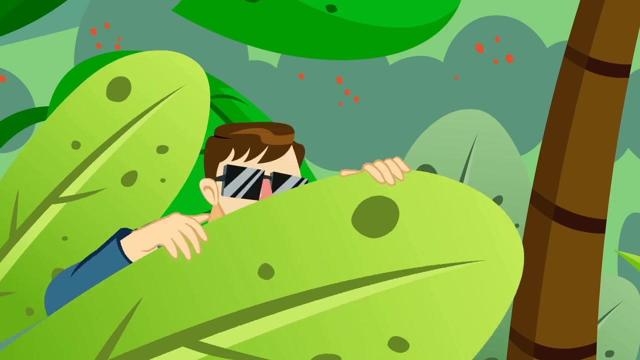 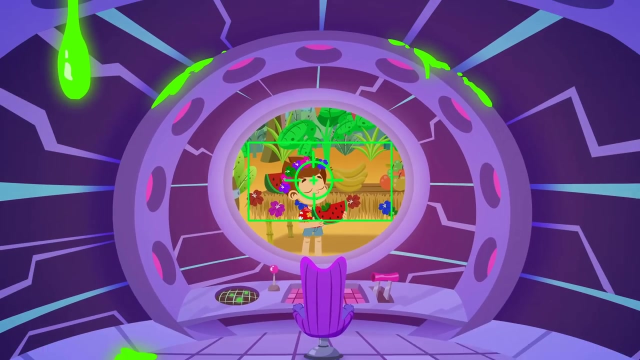 But we still need to clean up one more little thing. Bon voyage, See you next time. Today we're having a Hawaiian party. What a great plan: Music friends, a nice piece of fruit and Minions. Of course, Dr Spooky couldn't miss it. 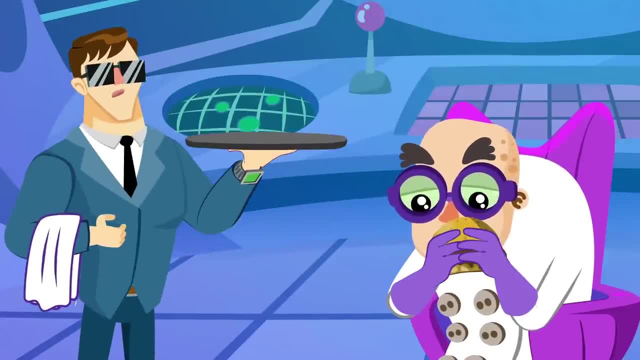 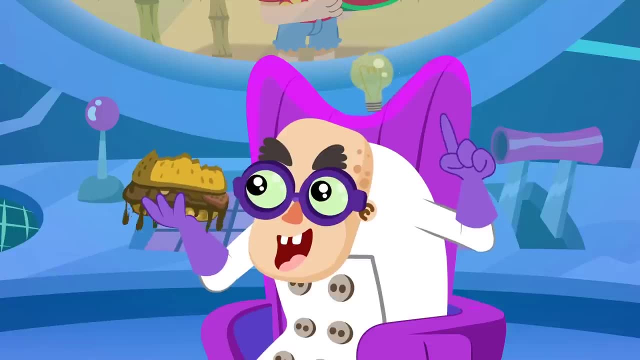 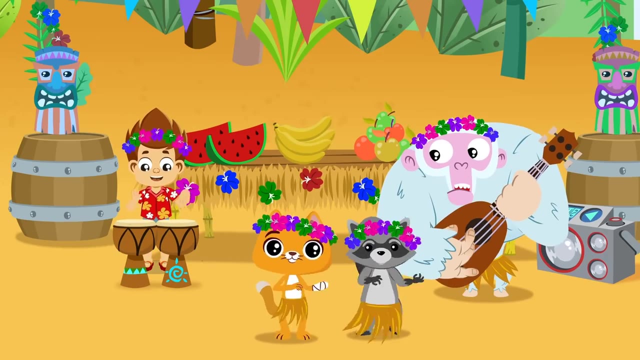 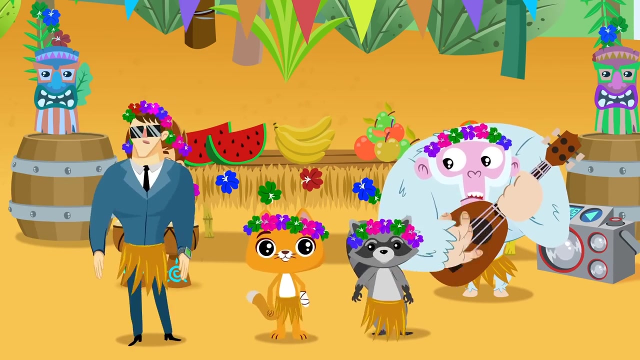 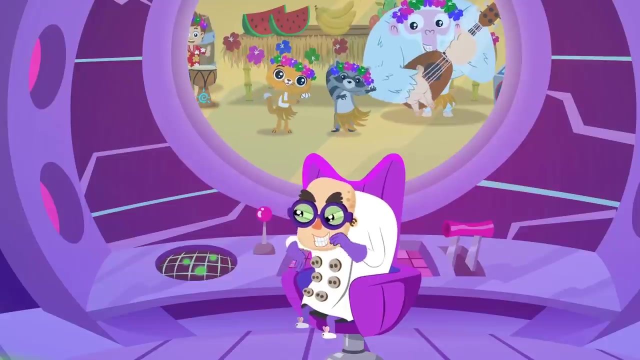 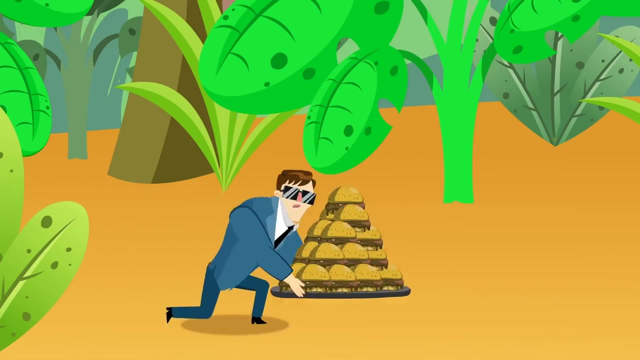 Yuck, What a nasty, greasy hamburger. Of course, A new evil idea. What A dancing minion. Is this your plan, Spooky Ha-ha? Wait a minute. Where did that giant tray of hamburgers come from? 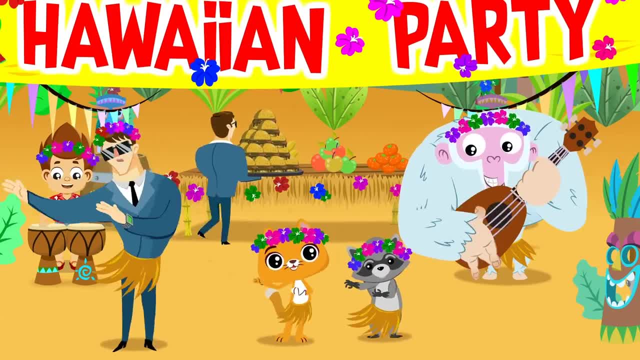 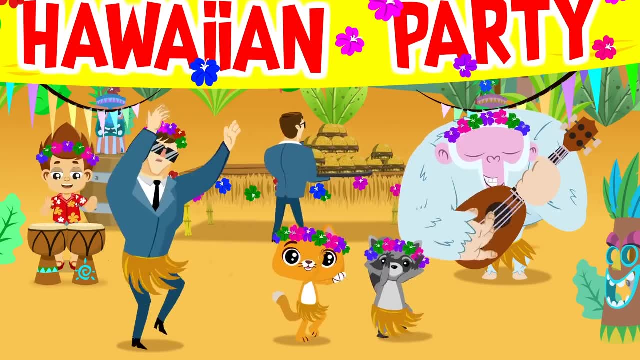 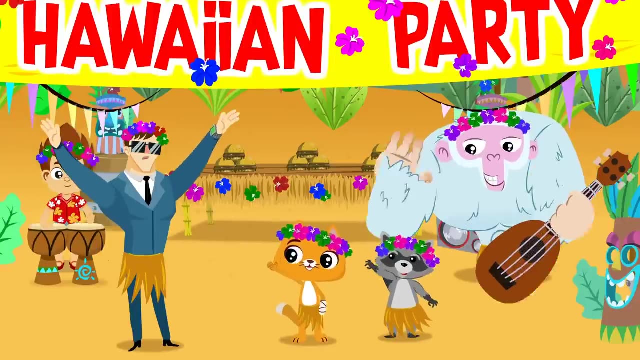 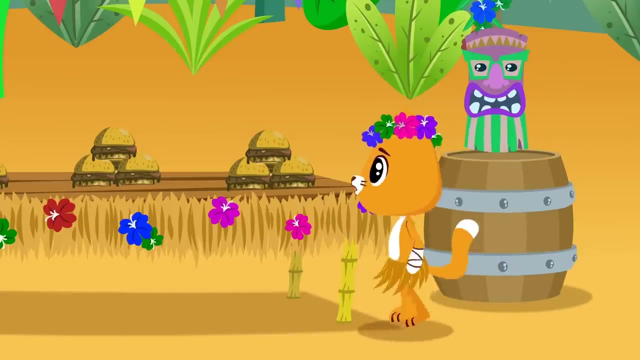 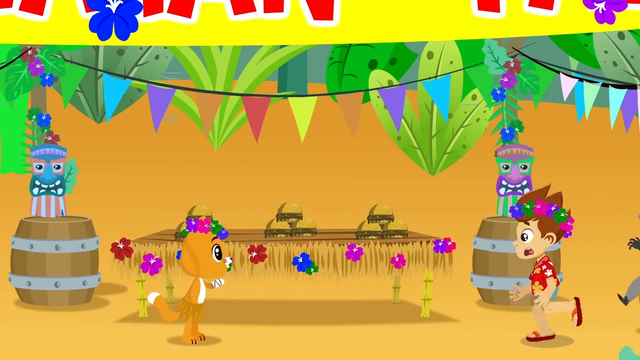 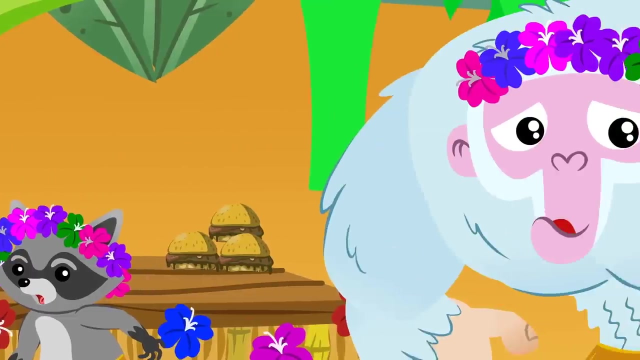 And what are you guys going to do with them? The minion is tossing all the fruit And putting the hamburgers in its place. Oh no, Dr Spooky ruined the party And on top of that, we are getting hungry. 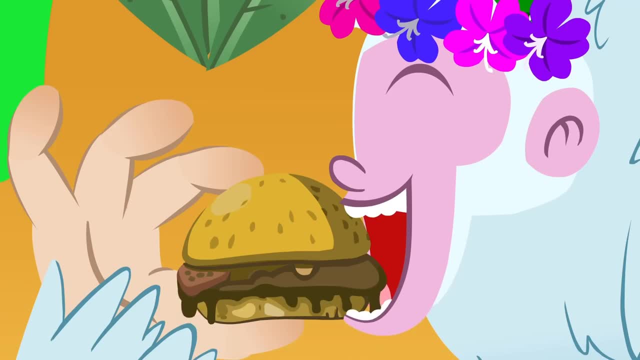 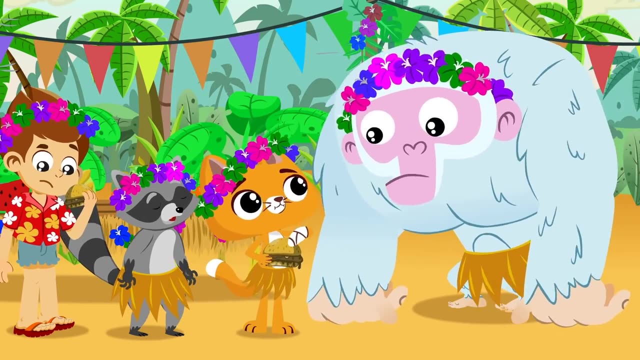 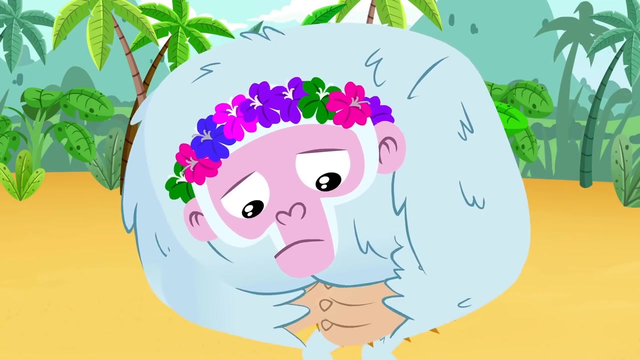 No Monkey Resist it. Don't take a bite of the hamburger. Phew, That was close. There's got to be a way to eat something that's not those horrible, horrible, horrible, horrible, horrible hamburgers Aha. 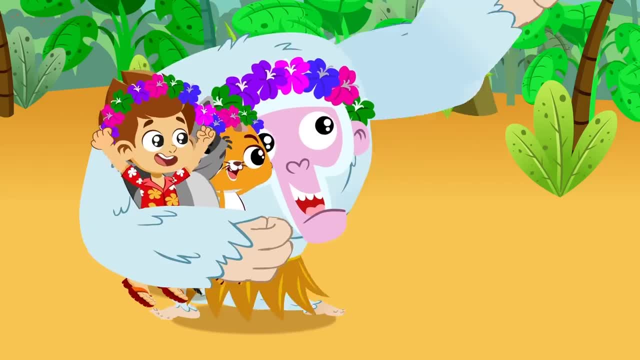 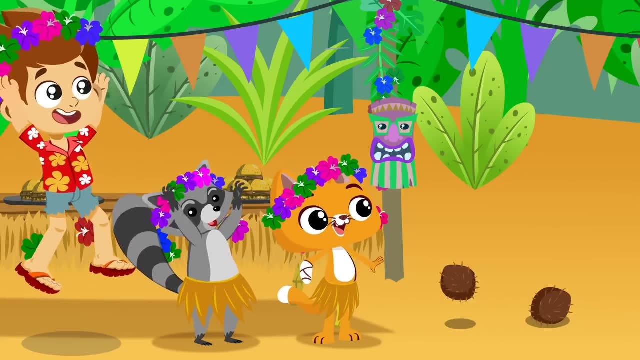 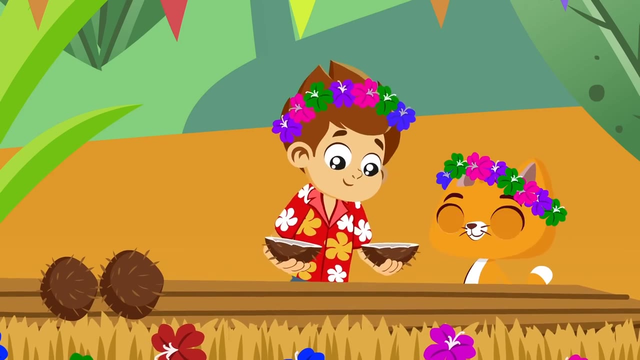 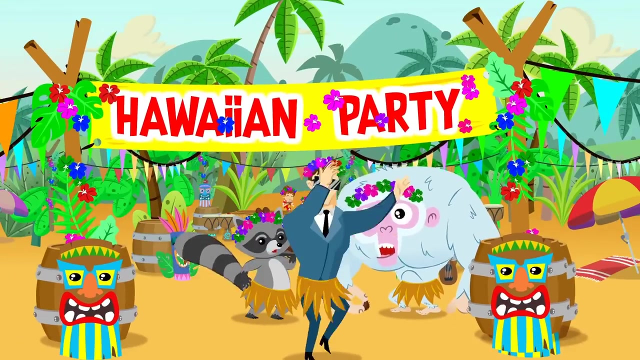 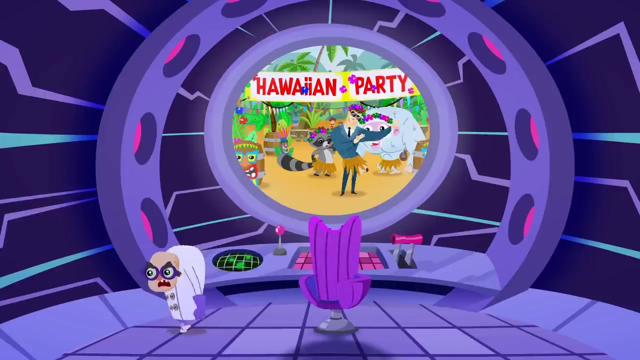 Coconuts. Monkey loves coconuts And he's really good at getting them from the palm trees. Yummy Coconuts for everybody, Everybody. The minions can have some too. You lost again. Everyone is enjoying the party again. 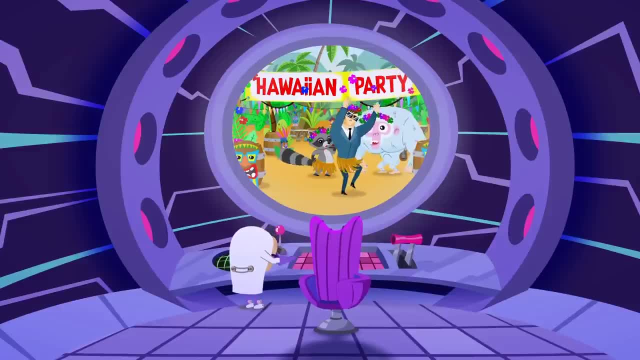 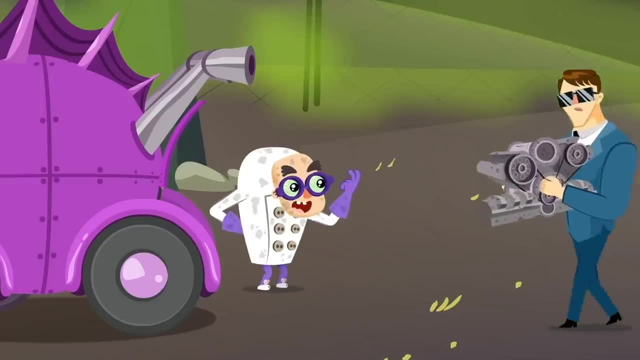 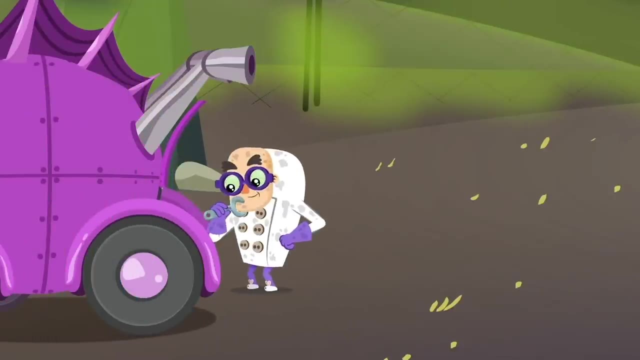 Dr Spooky, Your minion can't stop dancing. Oh well, What is Dr Spooky doing? Hmm, Oh my gosh, What is he doing? What is that? I've never seen anything so greasy and disgusting. 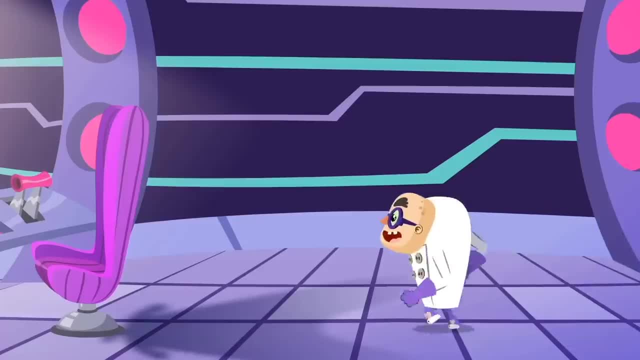 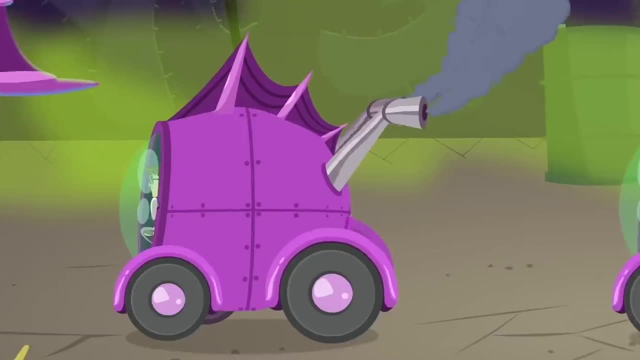 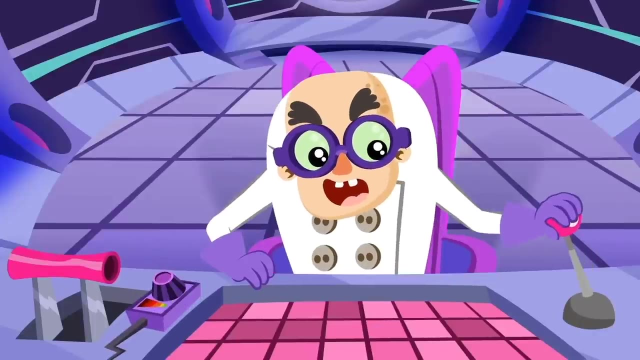 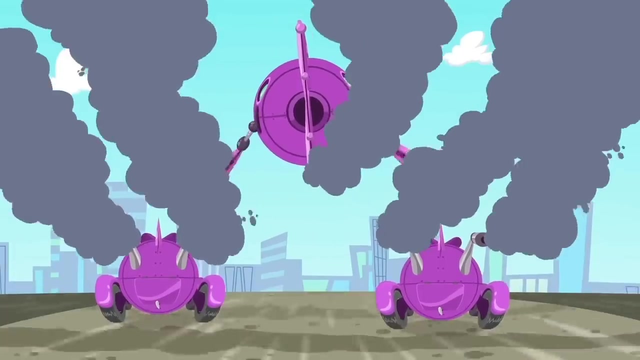 Now what? What's that remote control for Clack? The more he turns it, the more smoke comes out of the exhaust pipes. Look at all the pollution Dr Spooky and his gang are causing, and now they're going to cover the whole city with their horrible toxic clouds. 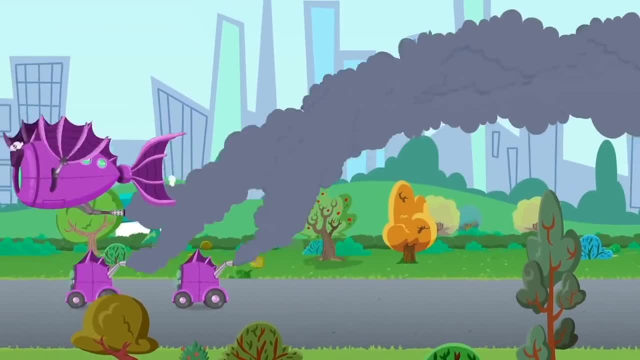 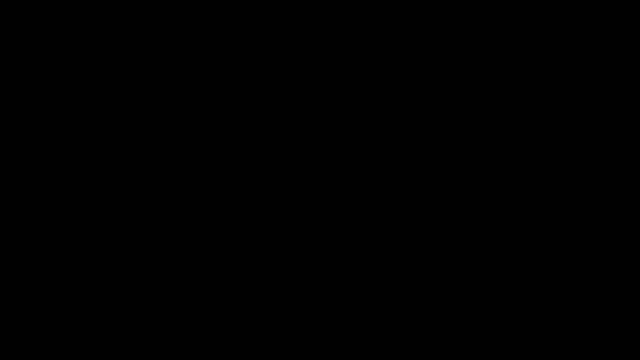 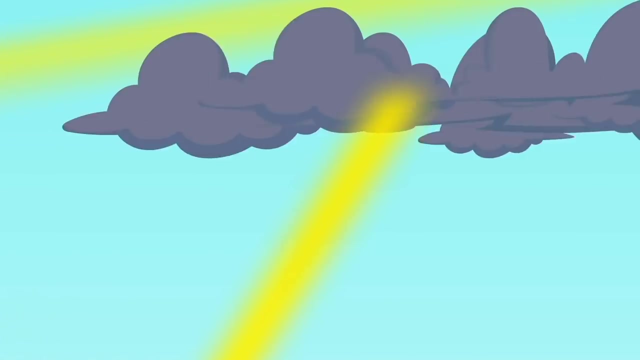 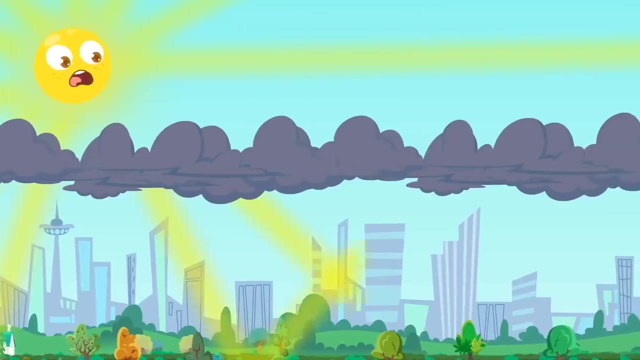 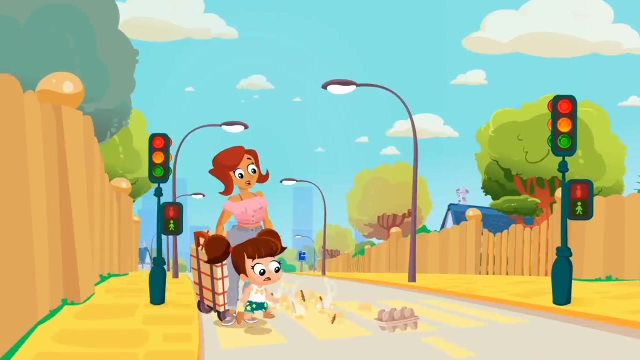 this is terrible. the whole earth has been covered in smog. the cloud of smog prevents the sunbeams from bouncing back out to space and they're getting trapped, and that makes the temperature rise. it's so hot that eggs fry in just a second and forget about eating ice cream. global warming is here already. 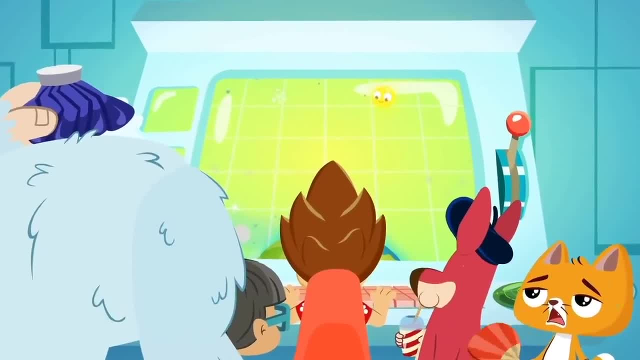 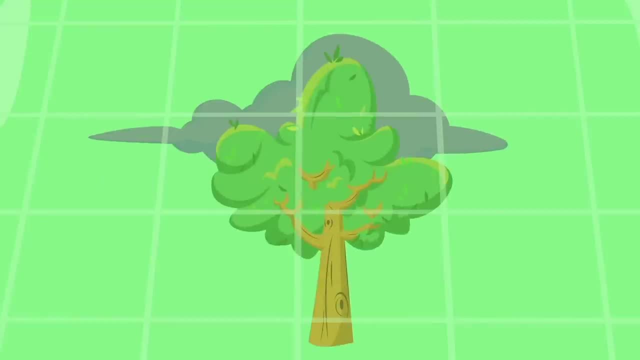 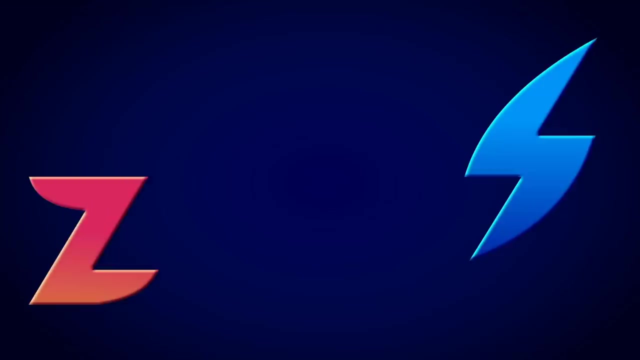 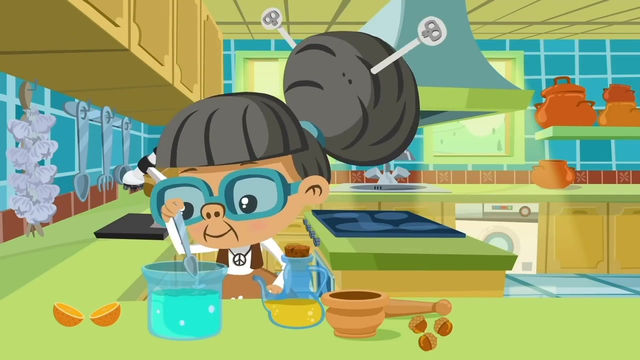 please, super zoo team, help us. we have to do something. aha, the trees can absorb the smog coming from the exhaust pipes and transform it into clean air. so, once again, nature has the solution. come on, kids, it's time to make a magic potion. come on, wise granny, let's solve the problem. 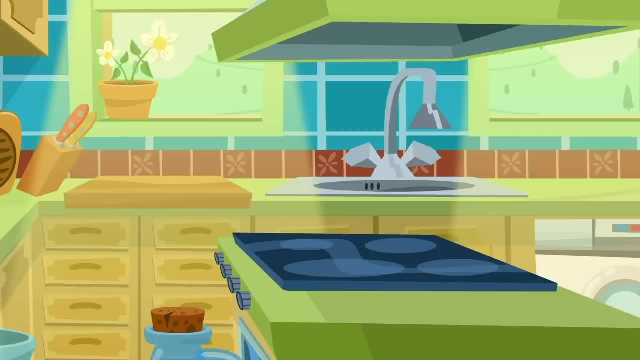 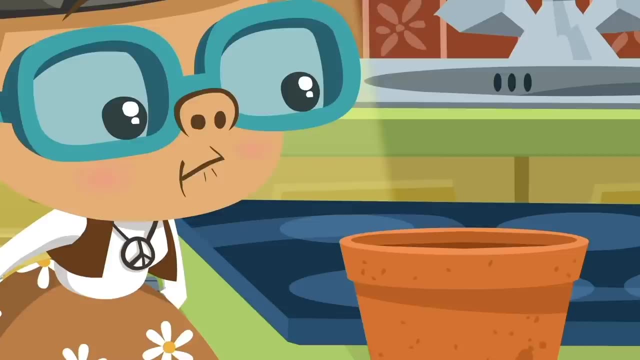 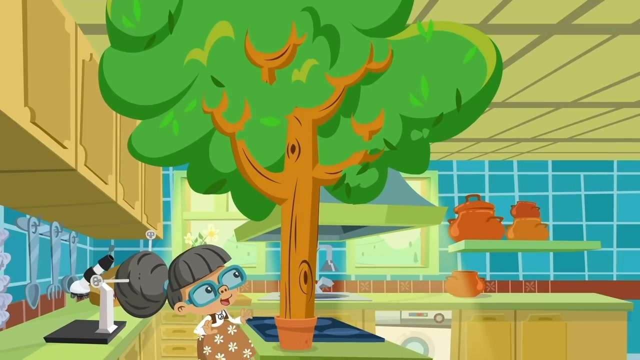 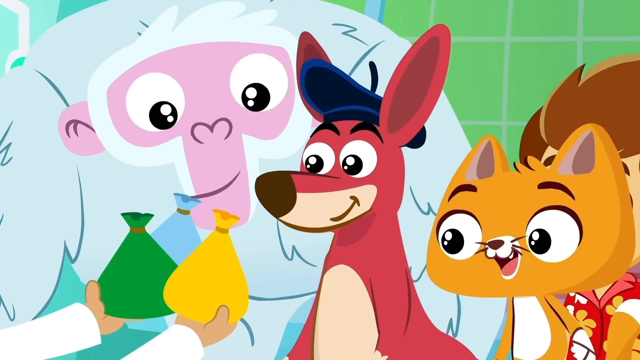 a little ultrasonic seed grower and a little sweet orange juice, of course. let's take a little bit of this mixture. uh-oh, it doesn't seem to work. it's too slow. what if we add a little more? wow, that definitely works. here are the super seeds. it's time to save the earth. to the transformation capsules. 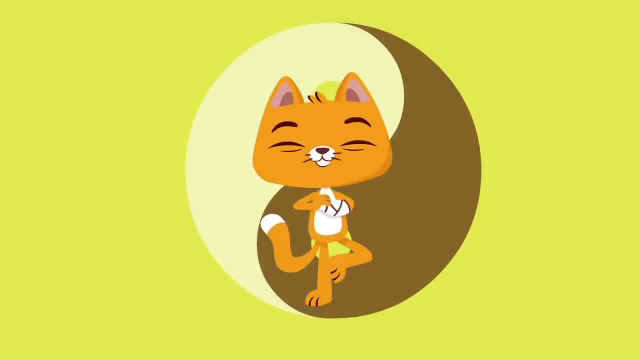 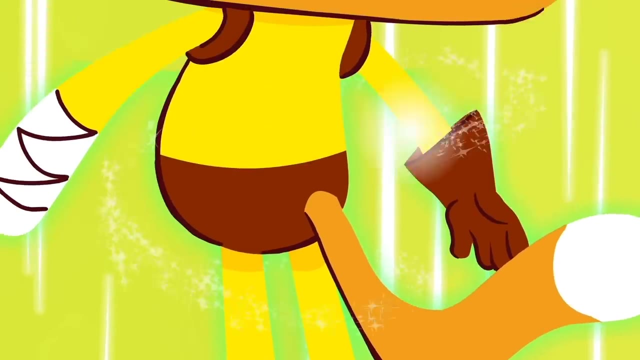 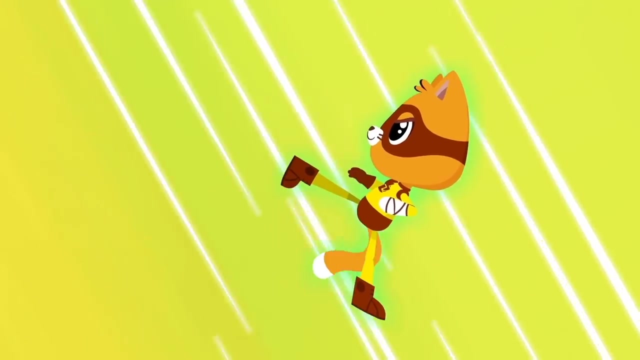 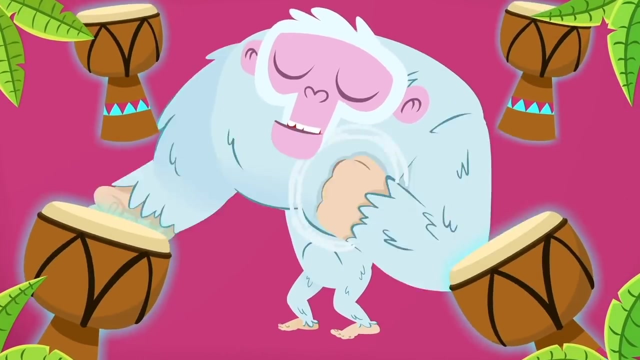 gotta walk the earth just to save the earth. it's the first step, and then it's the second step. we're moving like a dragon. all of a sudden, all of a sudden, someone's coming. I'm outside, I'm inside. there they are, here you go, look, look, look. 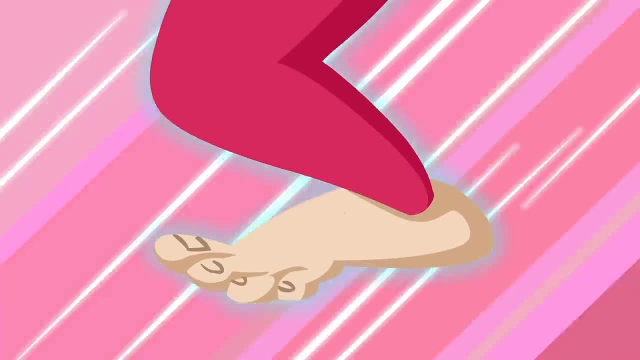 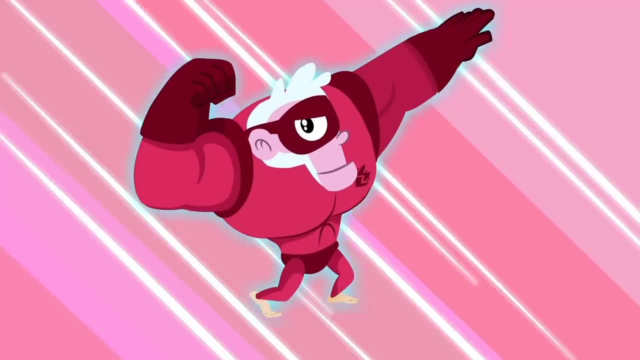 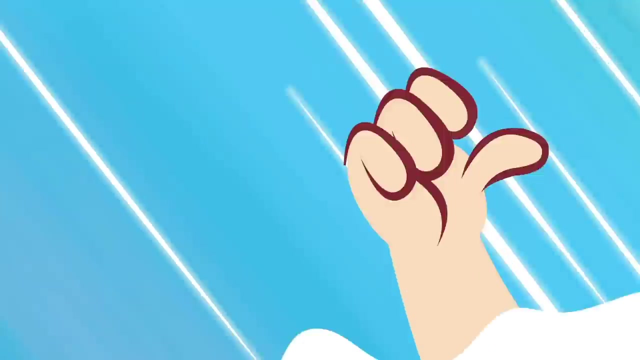 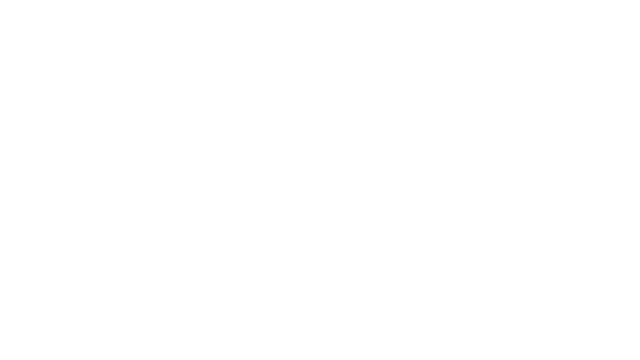 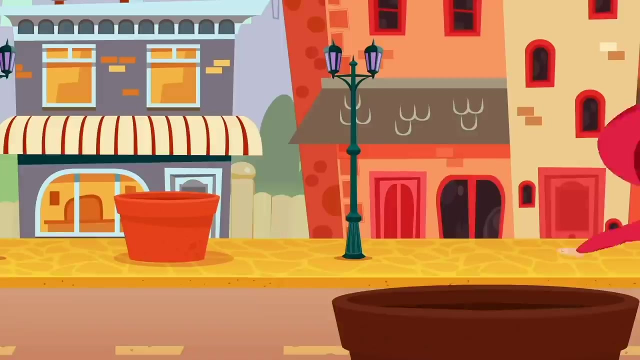 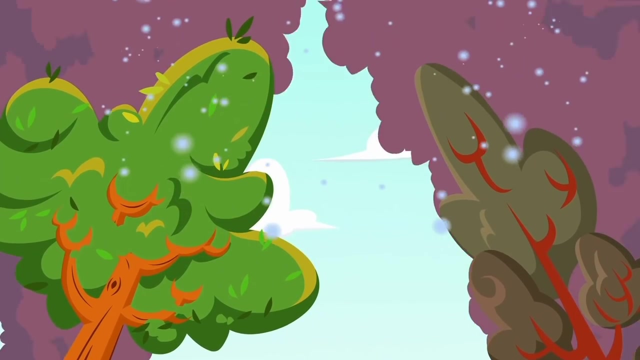 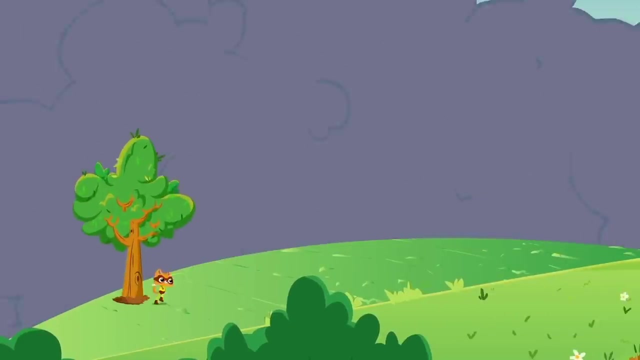 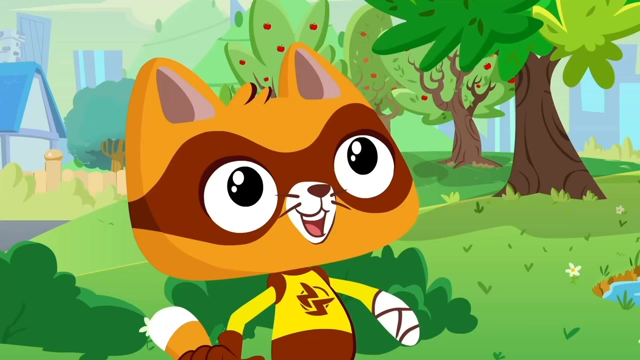 it's a big one. it's a big one. oh nice, Monkey, Kangaroo. Look how fast the trees that Catty and Monkey are planting grow. It's incredible. Look how clean the air is getting. Nature is wonderful, No matter how much Dr Spooky tries to pollute. 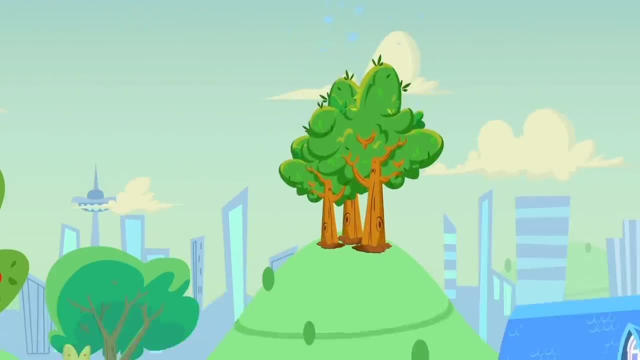 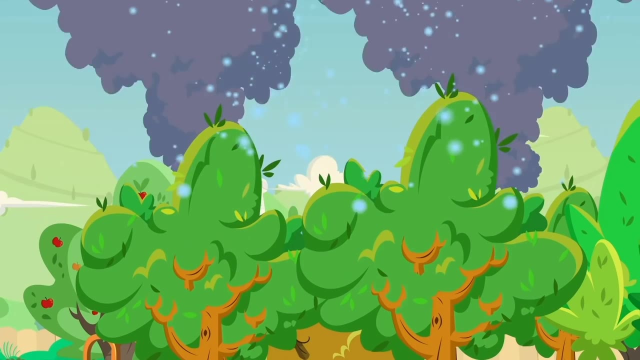 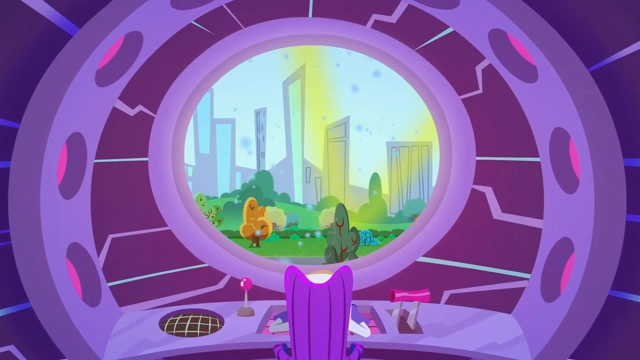 with the help of the Super Zoo team. the environment always wins. When we plant trees, we clean the air and leave the planet looking fantastic. It's so beautiful. Ha ha, Dr Spooky, the Earth is free from your disgusting pollution. 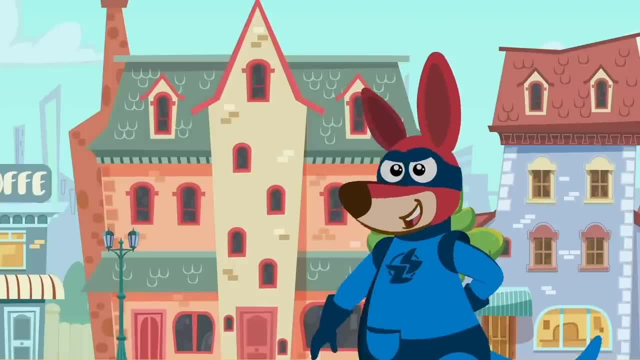 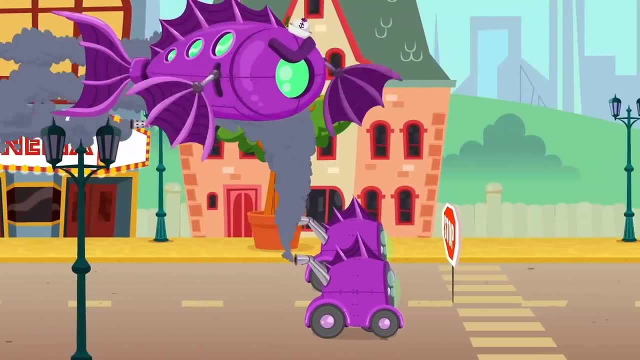 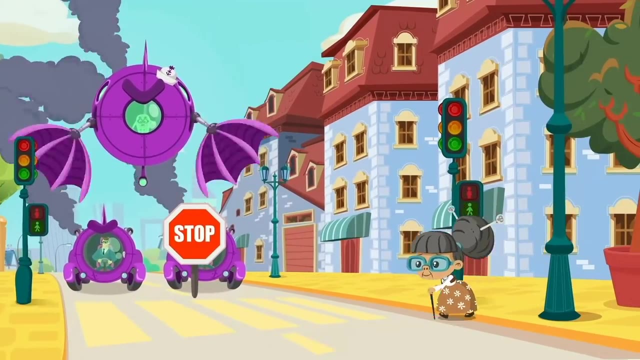 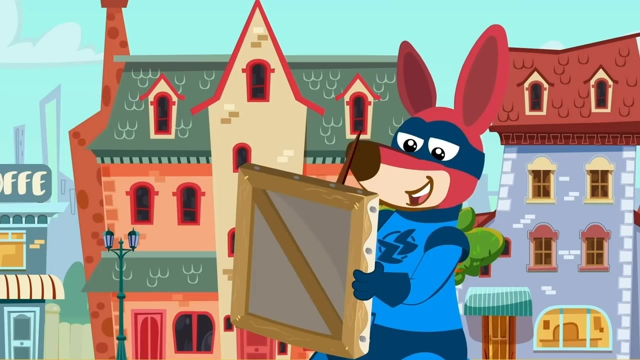 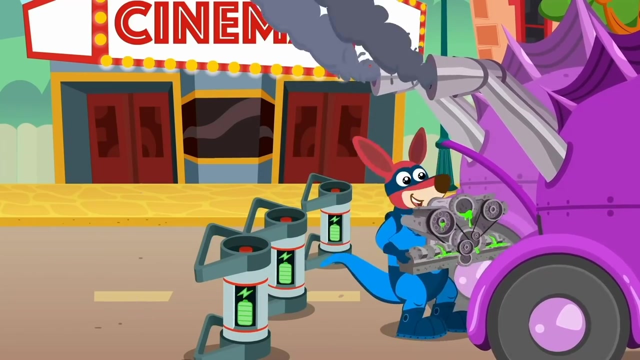 but you still have a lesson to learn. Stop please, You scoundrels. You need to respect the traffic lights. Hey, hey, hey, Take it easy. What a good idea: Kangoo Electric motors that don't pollute. 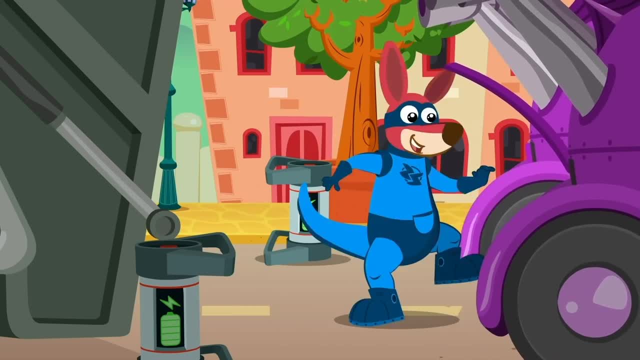 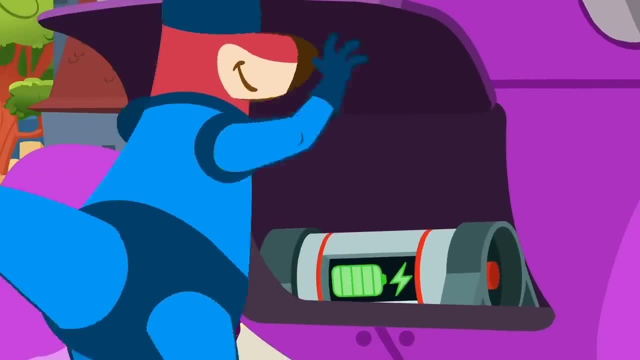 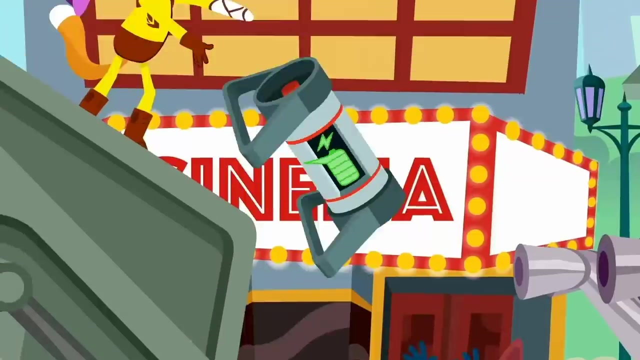 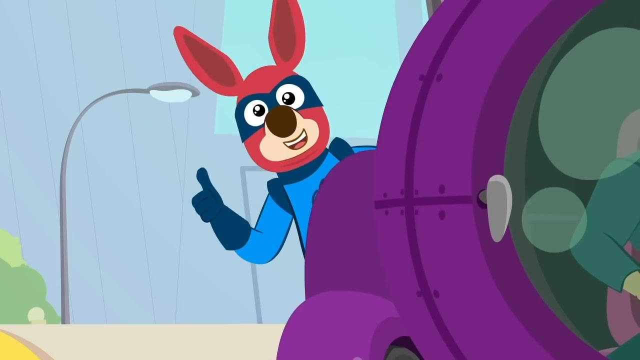 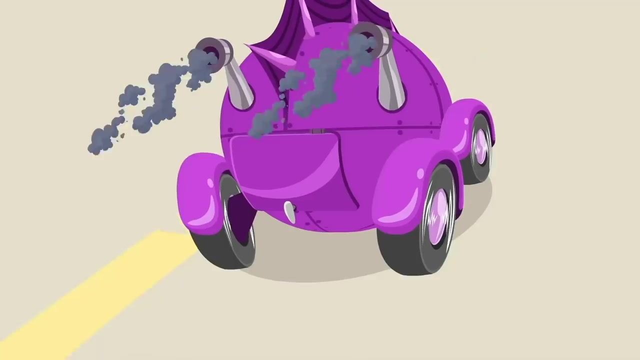 Bye-bye pollution, Hello, sustainable clean planet. Uh-huh, Hmm, hmm, Ah, Hmm, Ah, Ah, Great, Ha, ha, Ha, ha, Yay, Wow, No more long faces. Yeah, That's right, Dr Spooky, you're not seeing things? 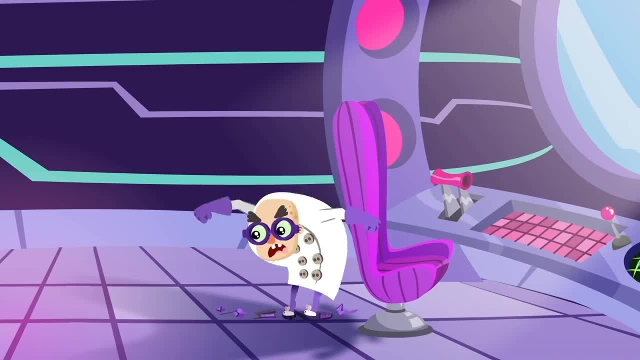 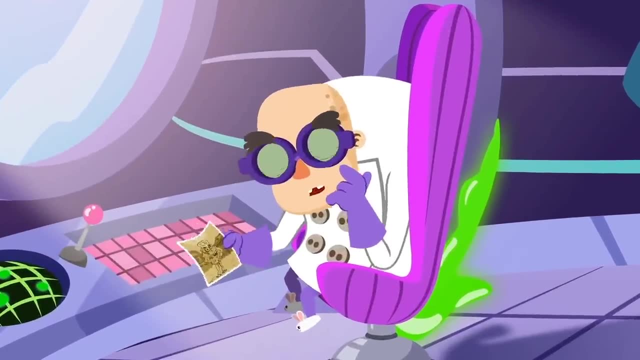 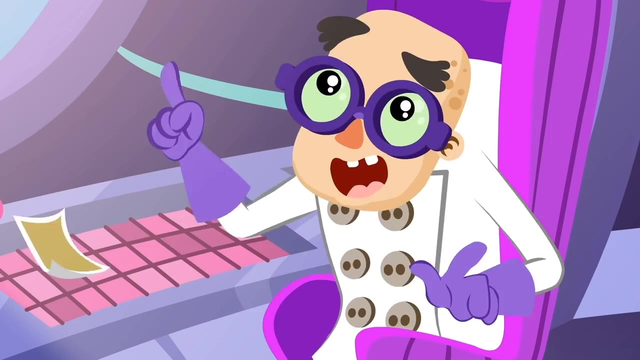 The Earth without those horrible clouds, the pollution is much better. Once again, we save planet Earth. Ha ha ha. Hmm, Oh, Dr Spooky, the bygone days always seem better. Uh-oh, someone has an idea? 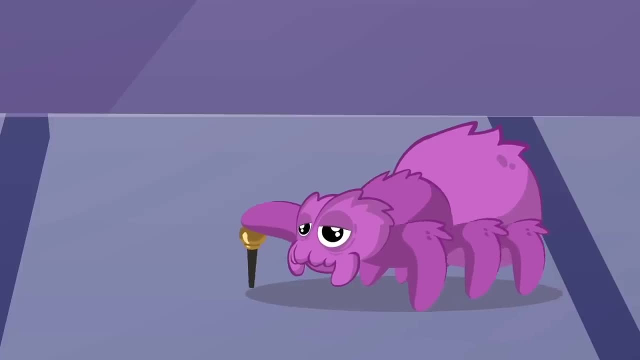 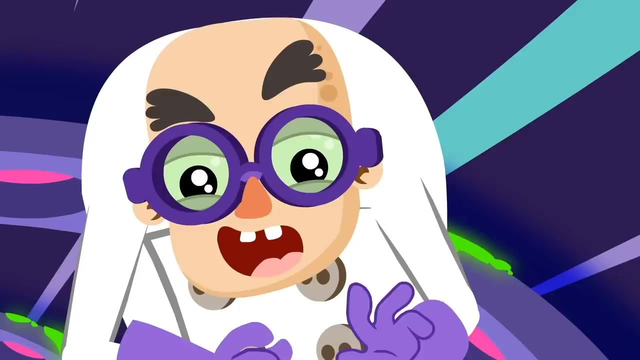 Ha ha ha. What a sweet old spider. Ha ha ha. We don't like Dr Spooky too much either. We'll wait and see. We should never be scared of him Like a little spider. I think Let's just go. 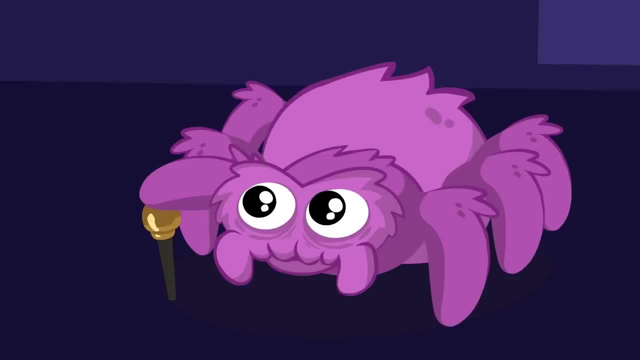 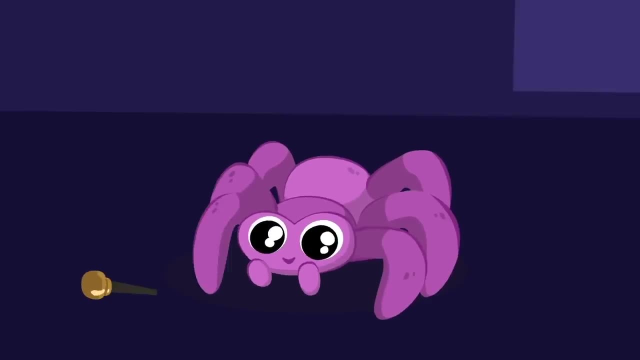 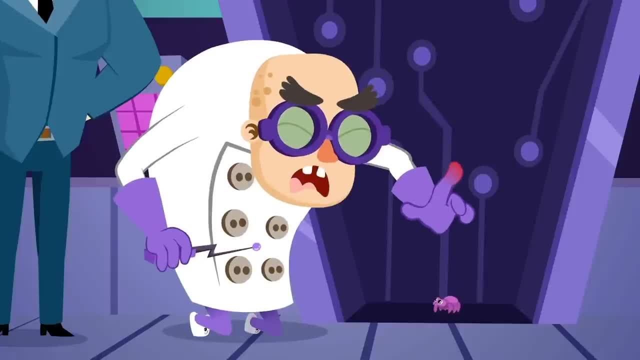 What the heck? The spider got younger. Okay, I think I see where you're going with this, Dr Spooky. Ha ha, Young ones know how to be rebels. Ha ha, I'm so excited, I'm so excited. 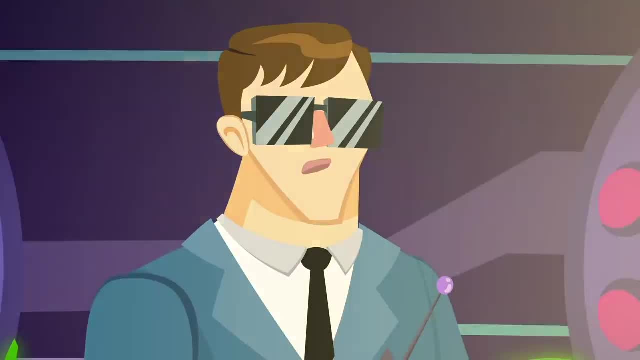 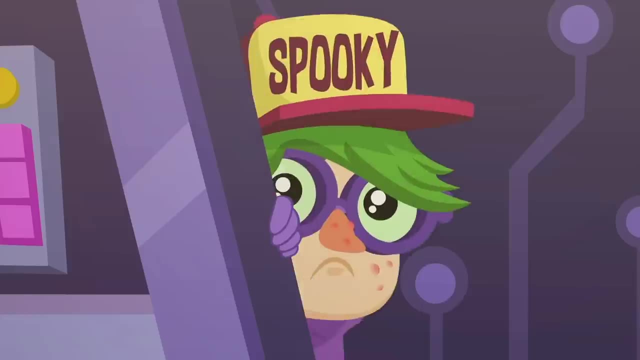 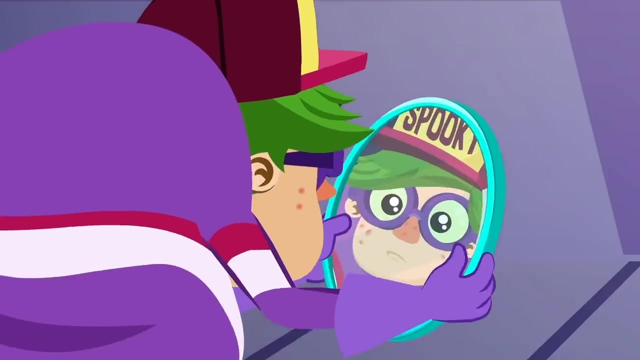 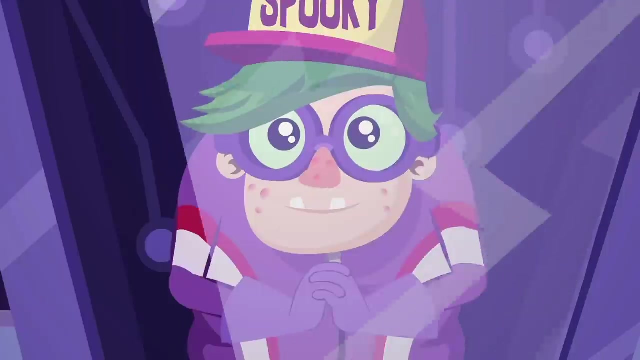 Let's see how well this invention works for Dr Spooky. I think you spun the wheel too far, guys. Should we try again? Wow, I don't think that. Oh well, if Dr Spooky is excited about it, let's see. 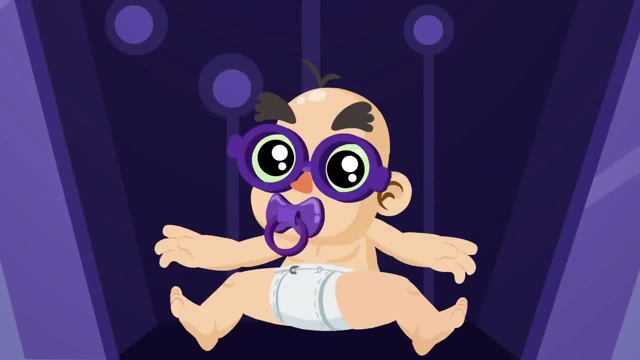 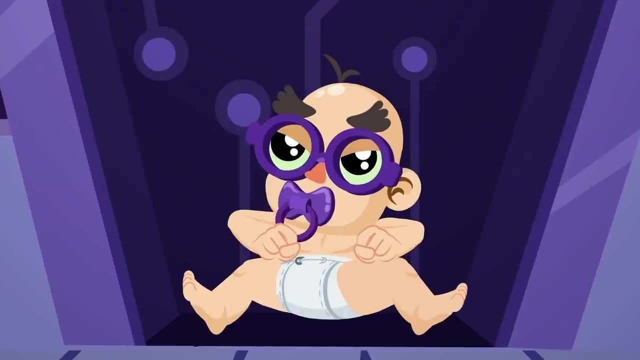 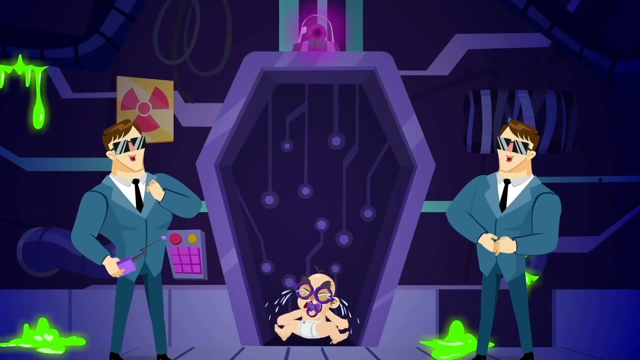 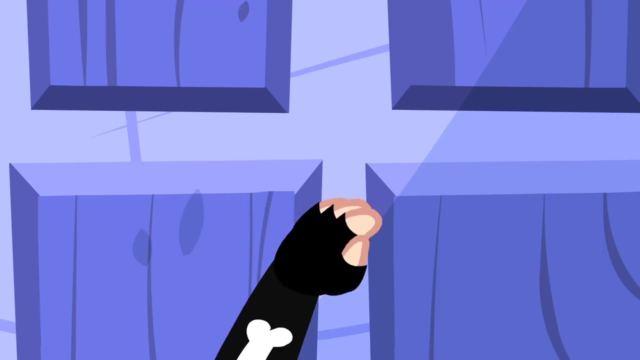 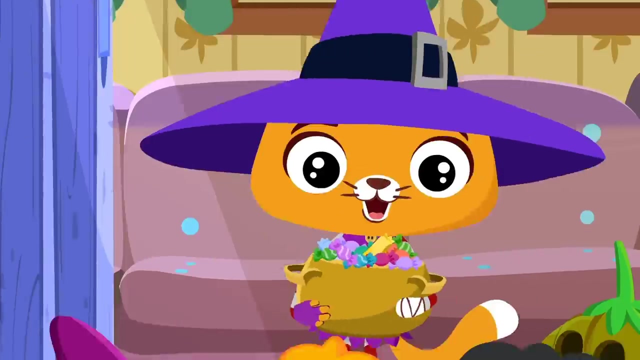 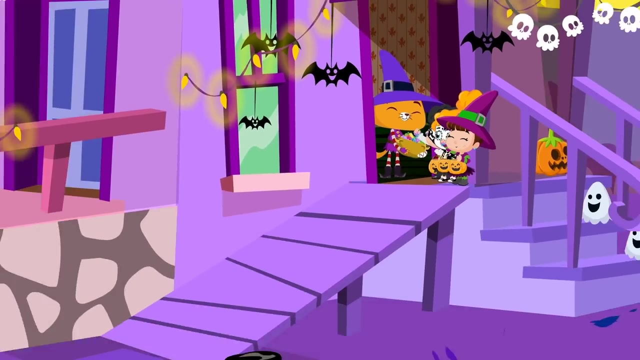 Is anyone there? I can't believe it. Someone's going to need a diaper change. Happy Halloween. Happy Halloween, Trick or treat, Catty Treat, of course. Uh-oh, someone is watching us. Dr Spooky wants lots of candy. 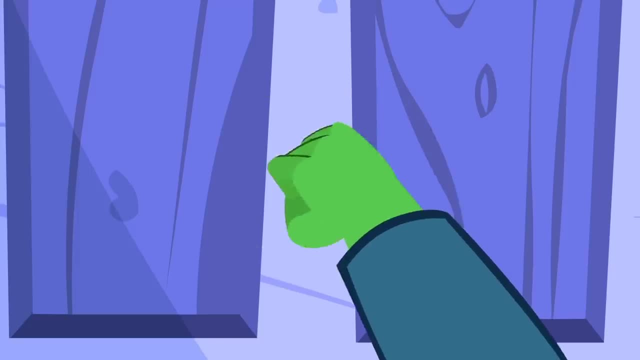 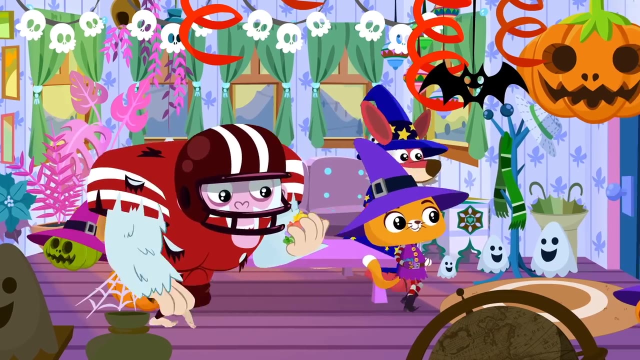 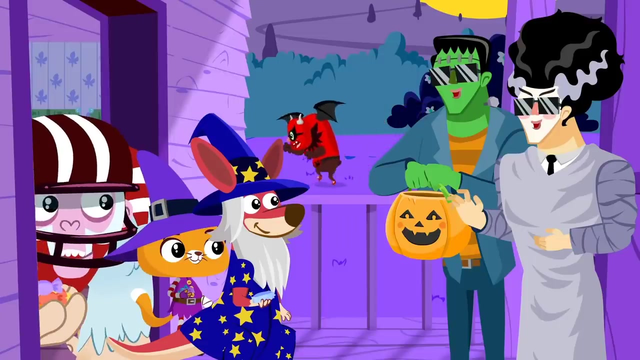 What are those costumes they're wearing? Well, the truth is, they're pretty funny. They're at the door, kids, And here they are, Frankenstein and his wife, And in the meantime, Dr Spooky is going through with his plan. 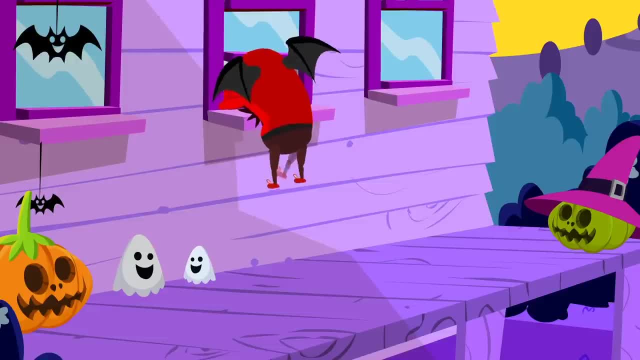 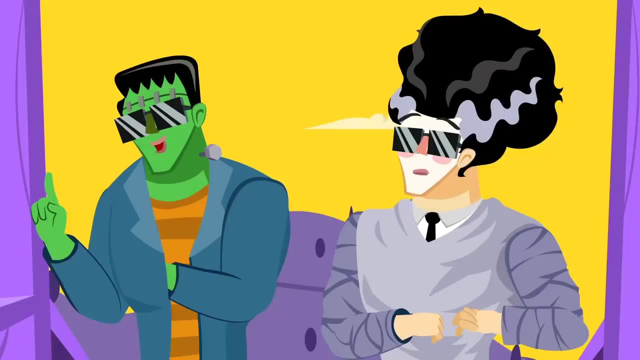 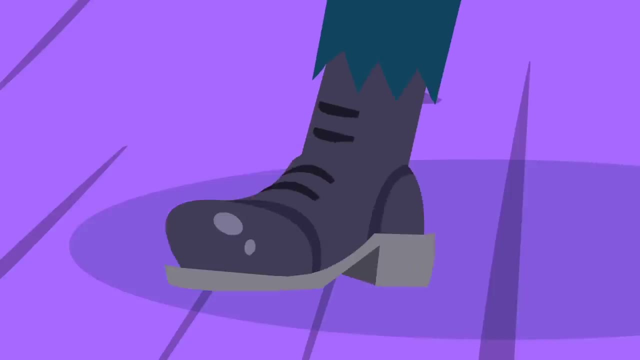 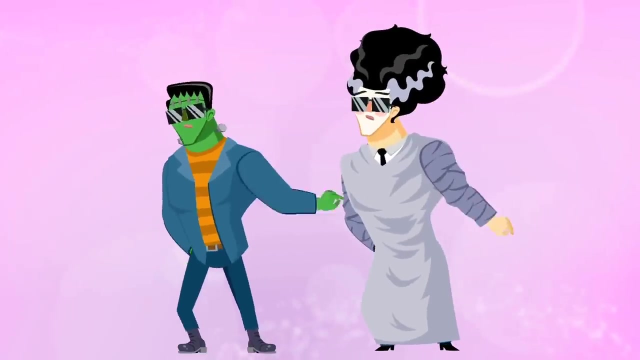 He's going to sneak through the window, But isn't he a little old for things like this? Dr Spooky is definitely seeing better. He's got better days. What's this spooker got there A radio, What? Well, let the show begin, I guess. 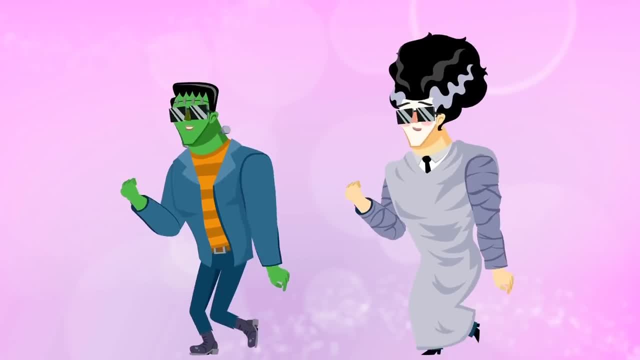 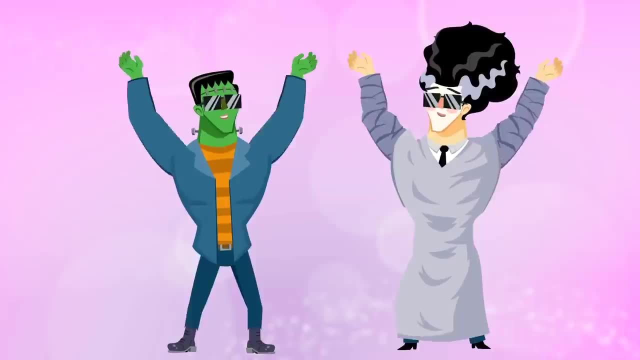 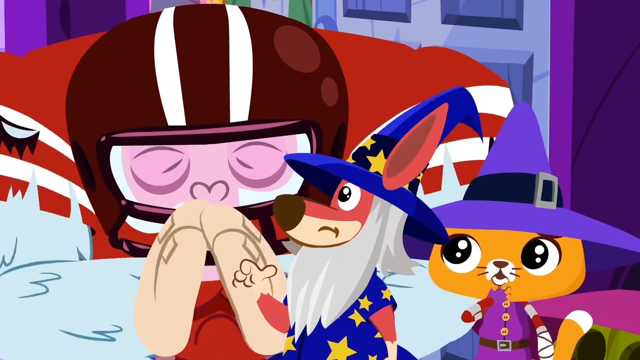 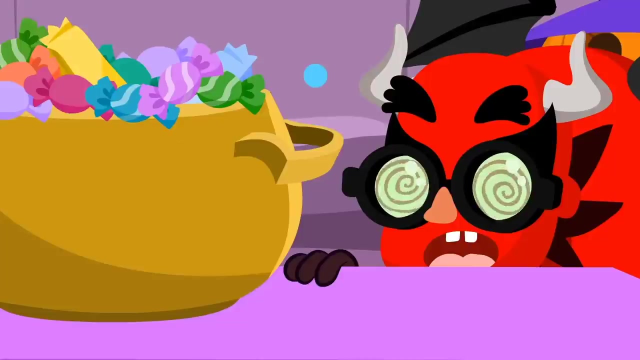 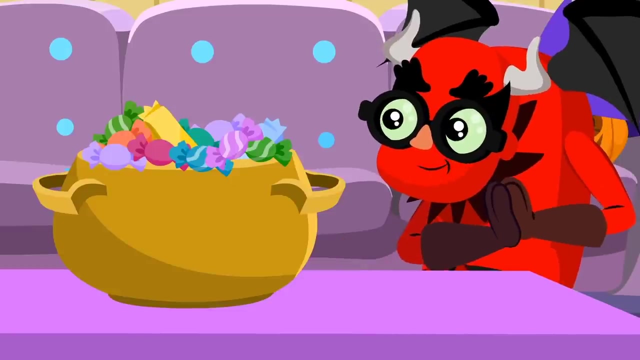 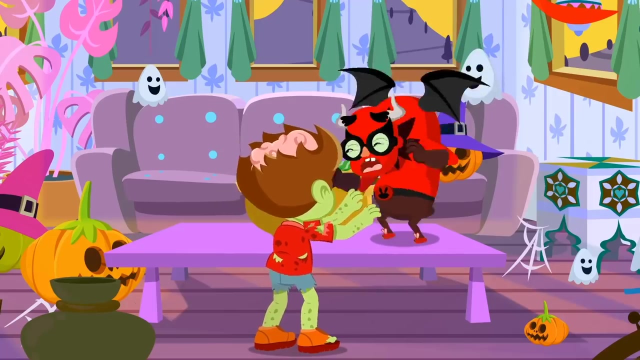 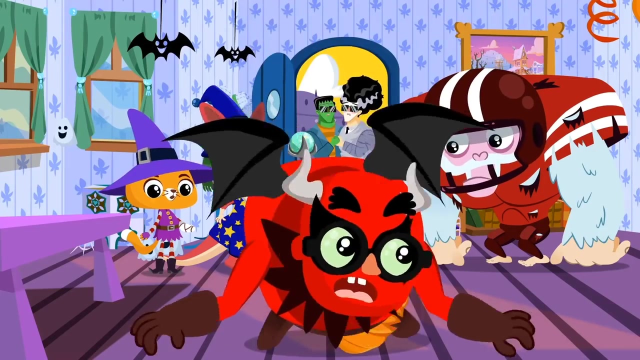 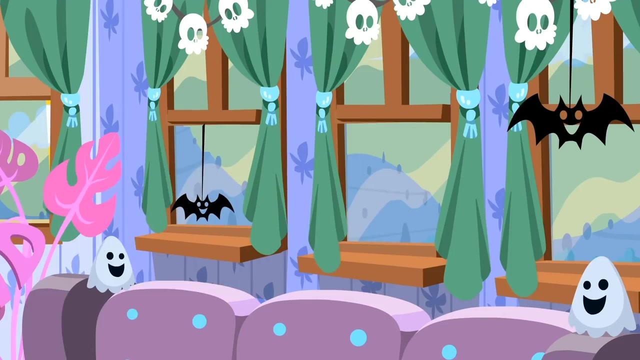 Hey Ron, Hey Ron, Hey Ron. what a show. and there goes dr spooky rolling like a meatball. that's a lot of candy. oh, he's going to grab it. watch out for the zombie. I've never met such a clumsy villain. 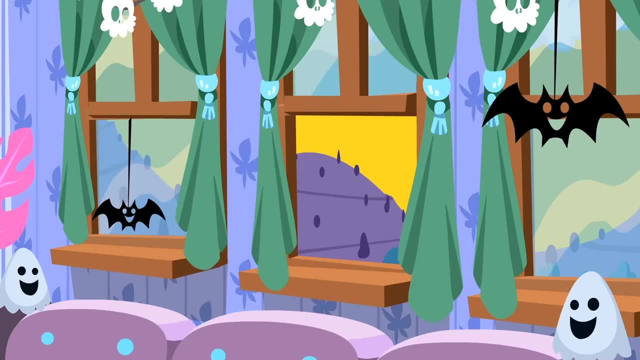 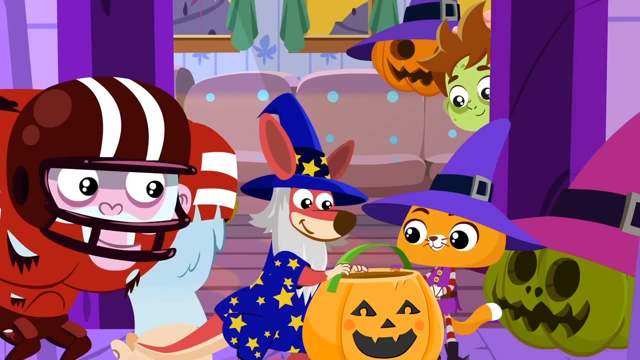 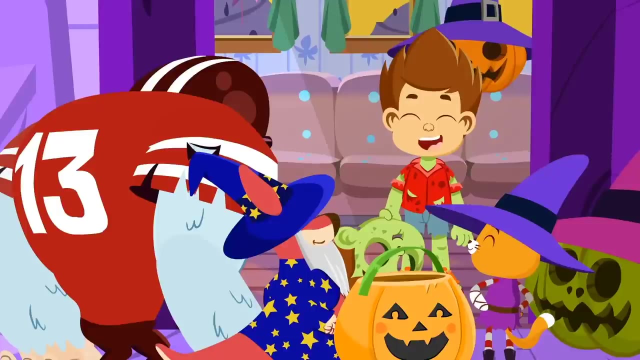 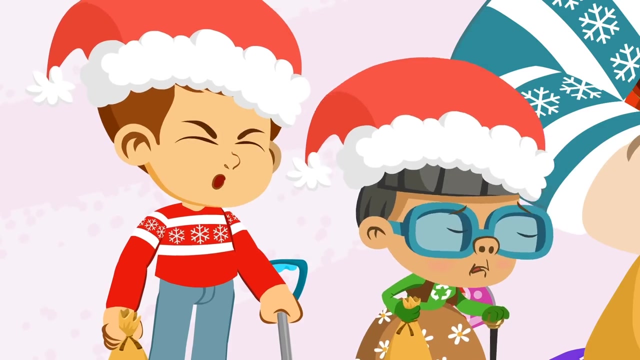 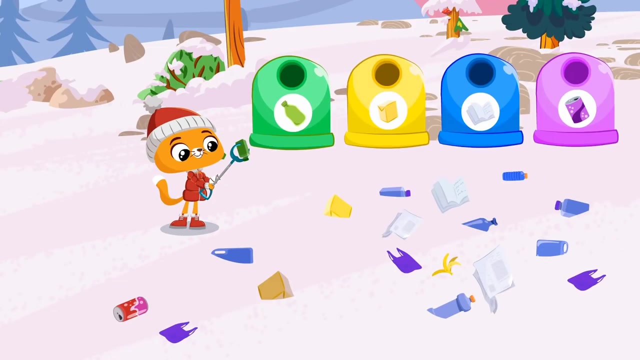 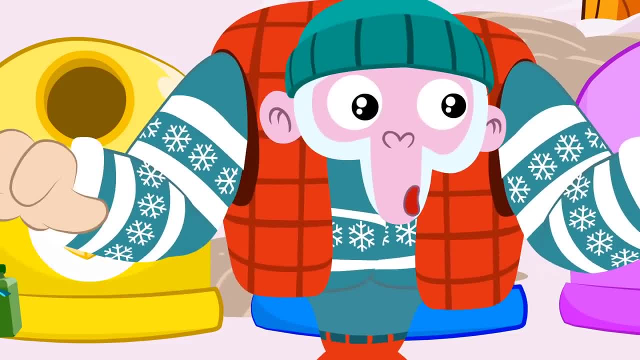 plastic. where does it go? I've got a bottle plastic. where does it go? I've got a bottle. where does it go? let's recycle the trash. where does it go? let's recycle the trash. where does it go? let's recycle the trash. the plastic comes in the plastic thing. 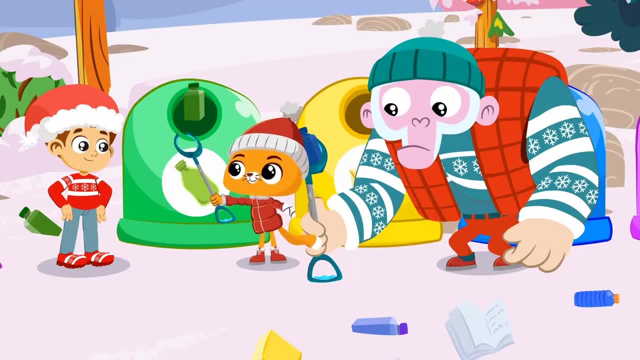 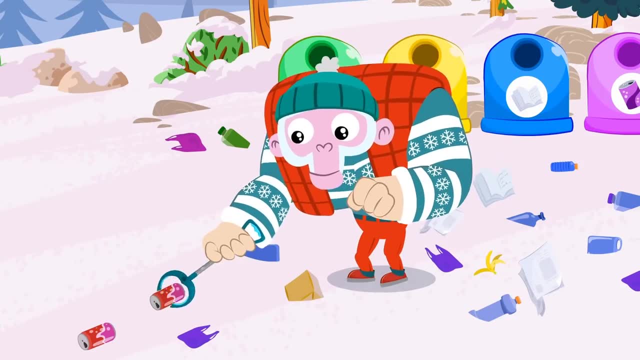 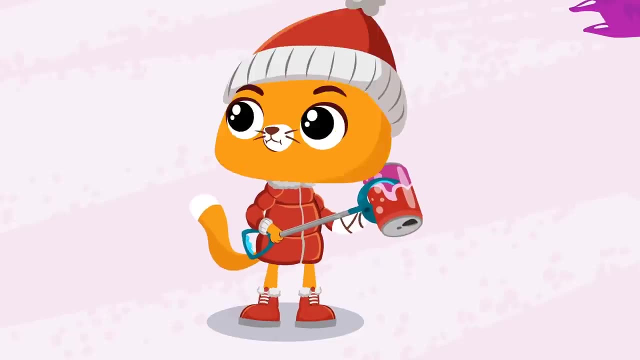 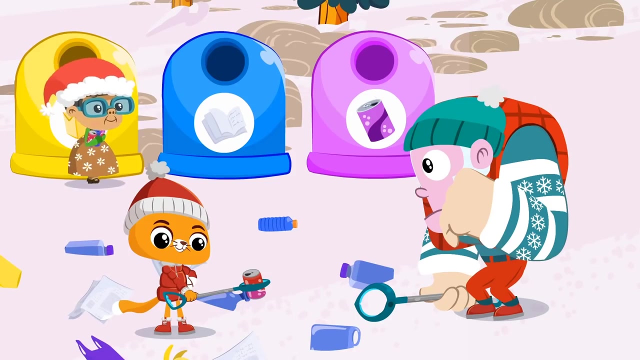 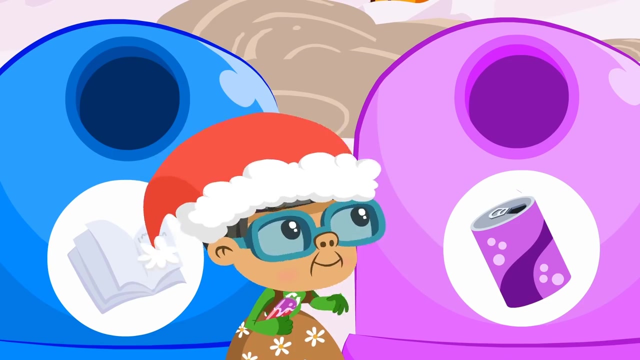 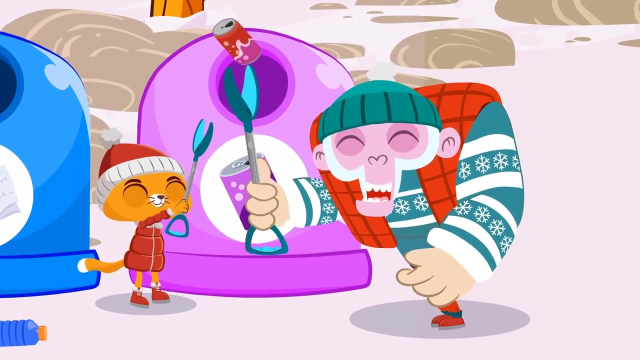 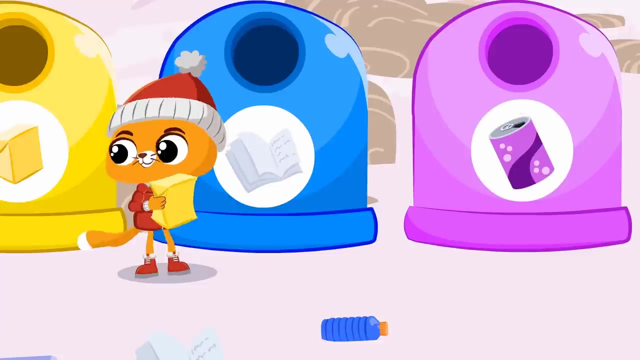 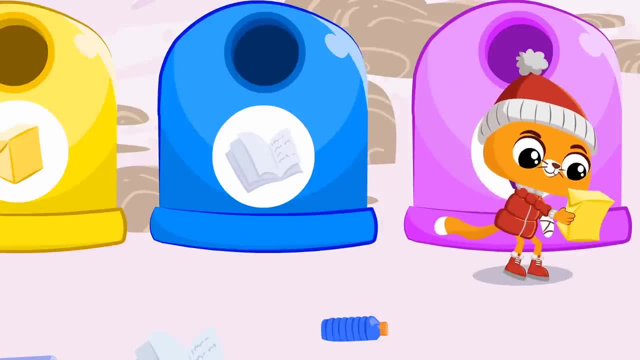 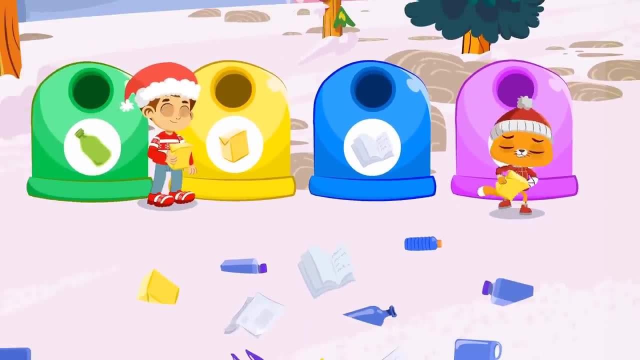 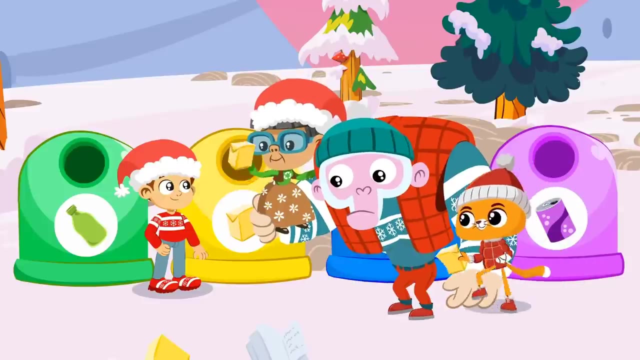 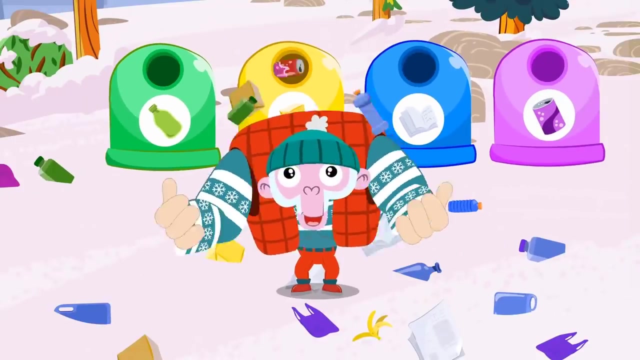 It's made of cardboard. where does it go? I've got a box- oh, where does it go? Let's recycle the trash. The cardboard goes in the cardboard bin. Let's recycle the trash. I've got a jar- oh, where does it go? 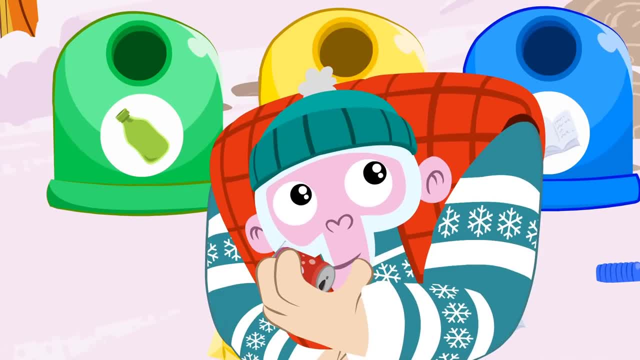 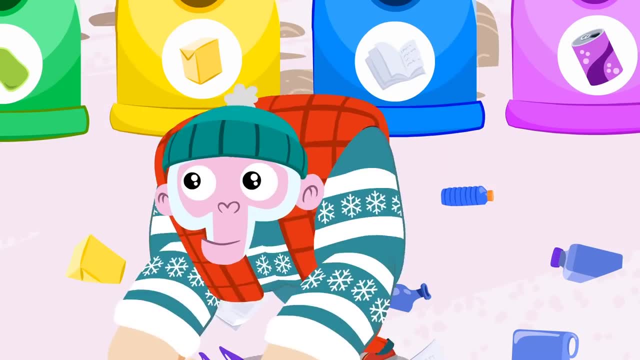 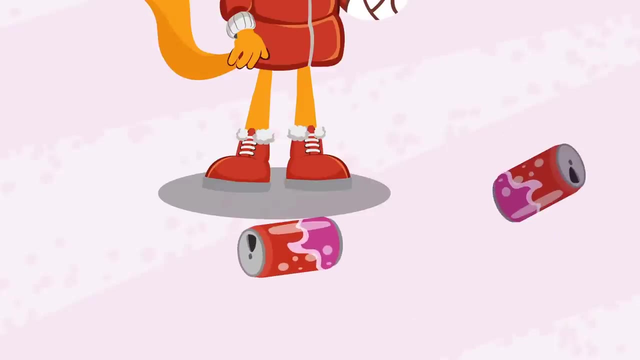 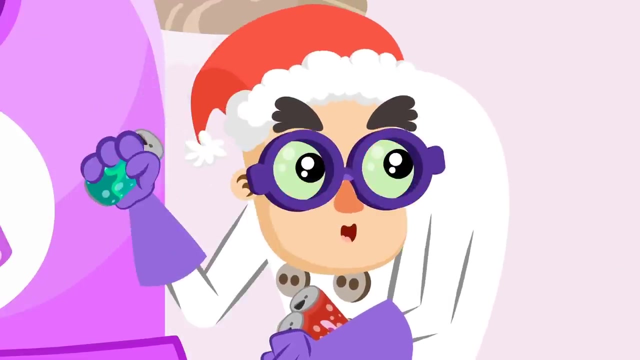 It's made of glass- oh where does it go? I've got a jar- oh where does it go? Let's recycle the trash. The glass things go in the glass trash bin. Let's recycle the trash. The mountain is clean. yes, thanks to the kids. 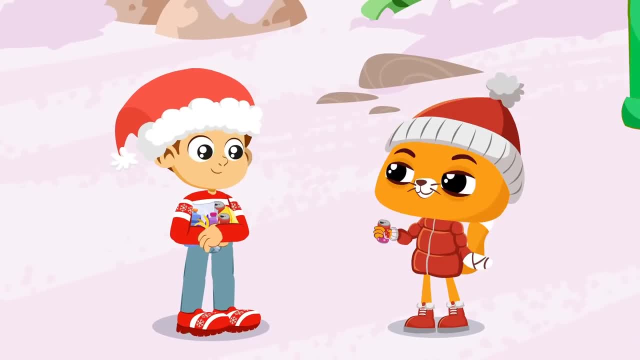 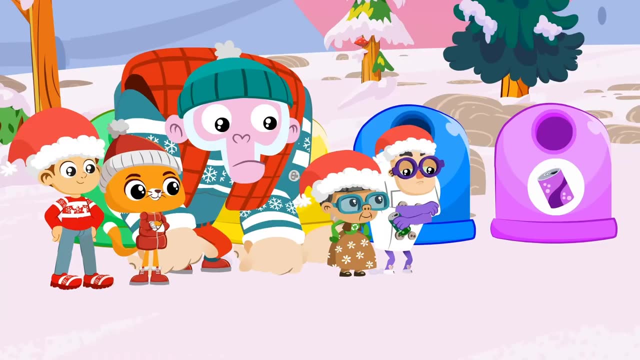 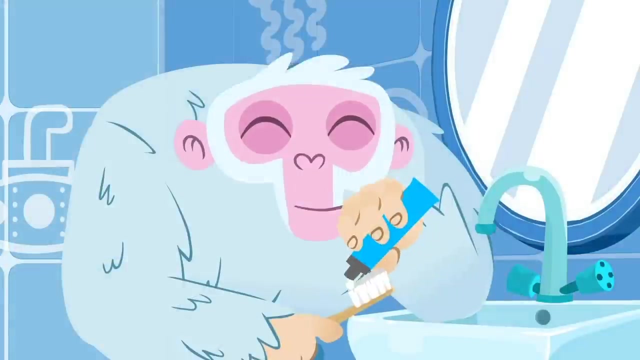 The mountain is clean. yes, thanks to the kids, The mountain is clean. yes, thanks to the kids, We've recycled the trash. We've recycled the trash. Welcome to Kids' Learning Corner. Today, we'll learn a new way to help the ecosystem. 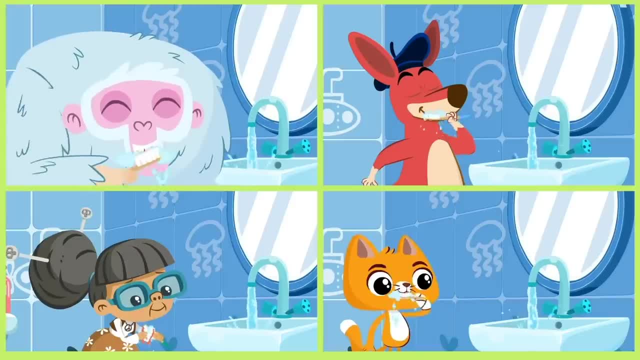 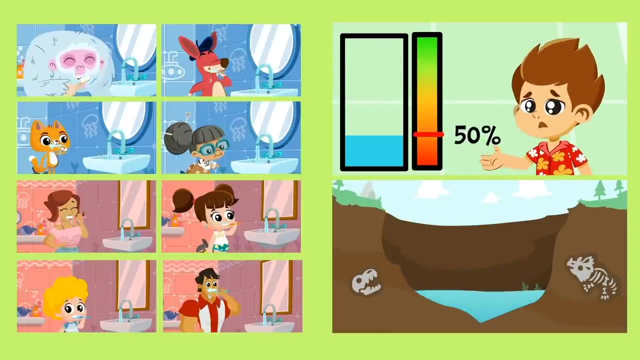 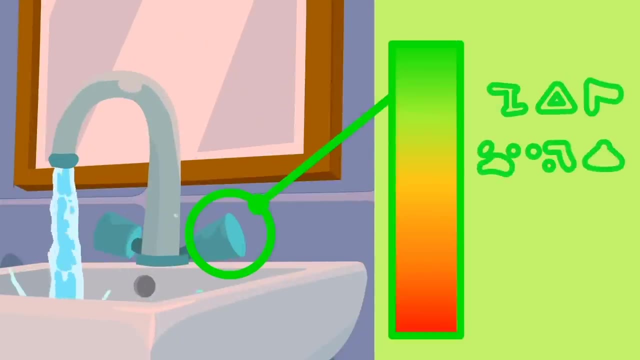 We brush our teeth every day, or at least we should- And sometimes, when we are brushing, we leave the tap running. We waste lots and lots of water this way. Hey, everybody With something as simple as turning off the water while we brush. 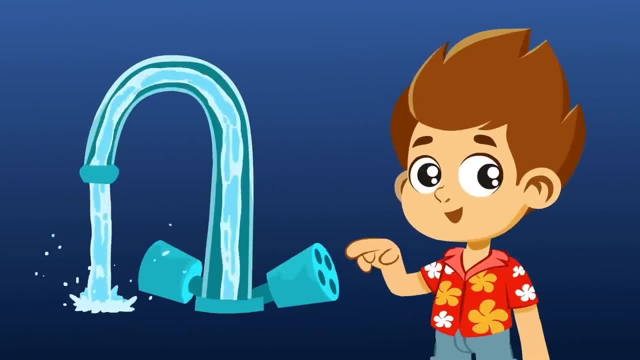 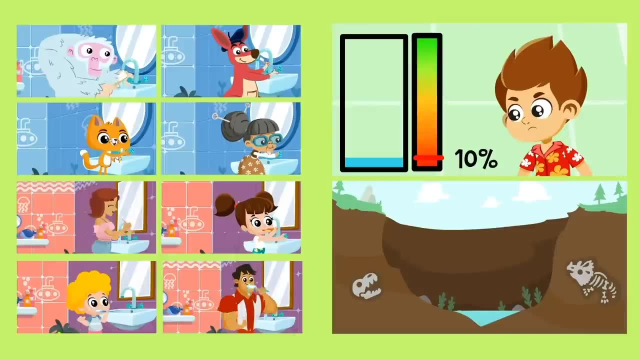 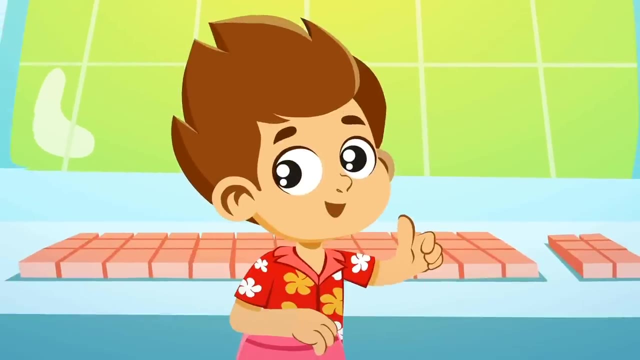 we can make the world a better, more sustainable place. That's it, kids. great. If we change little things in our day-to-day lives, we can help our planet. Let's save the environment together. Welcome to Kids' Learning Corner. 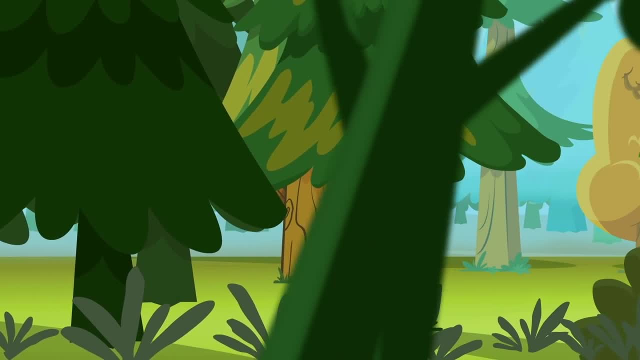 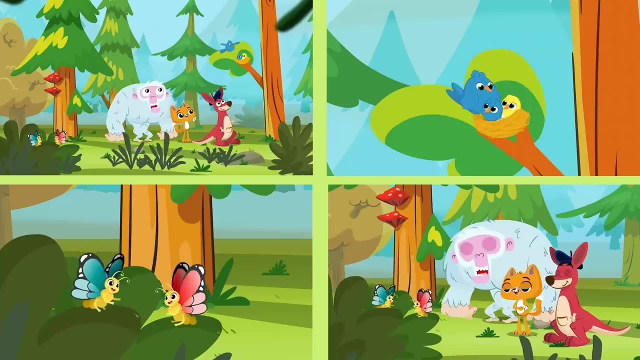 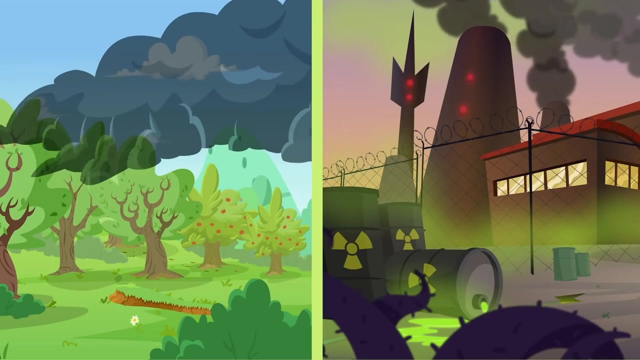 Today, we're going to learn about deforestation. The disappearance of plants is called deforestation. The trees are the shield that keeps pollution from reaching the atmosphere. Unfortunately, the levels of pollution keep rising and there are less and less trees. If there are no trees to keep the clouds of pollution in check, 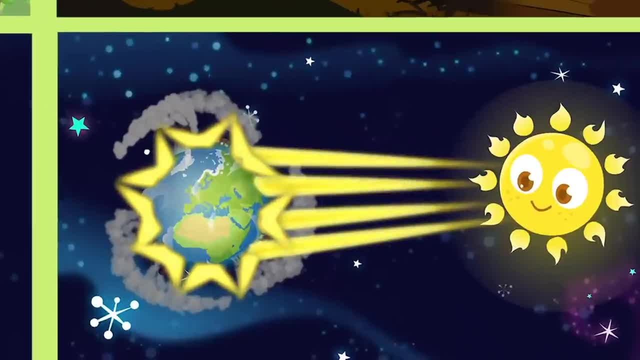 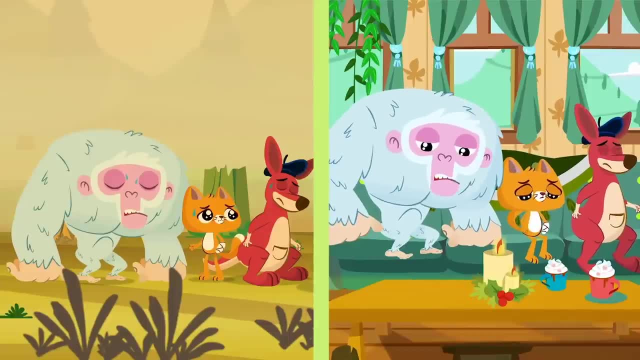 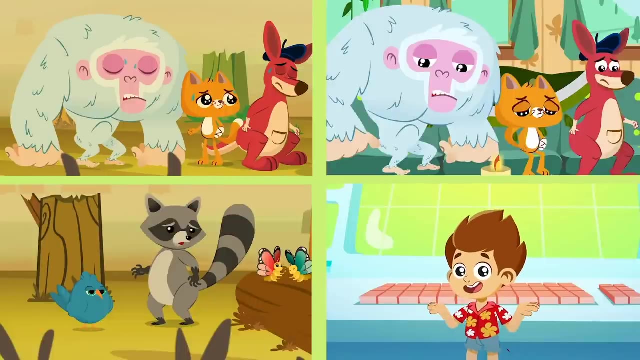 the sunbeams can't bounce back into space and are trapped on Earth. This is why the temperature is going up uncontrollably. Pollution makes us sick. Many living creatures also lose their homes when trees disappear. But it's not too late. 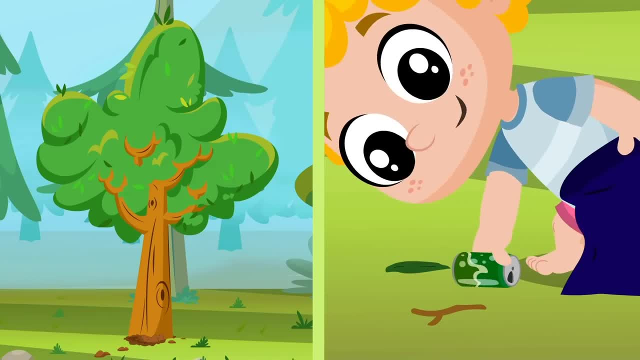 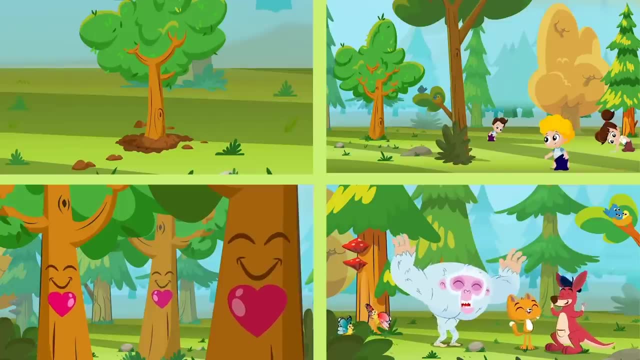 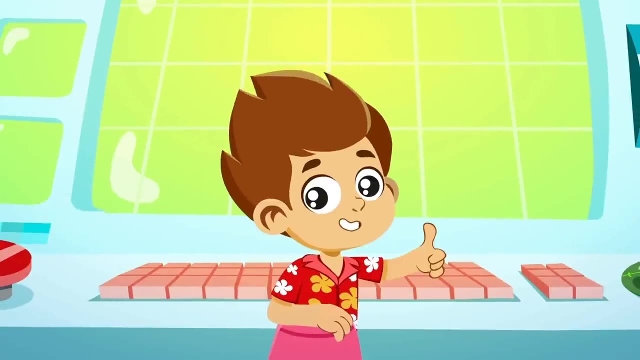 How can we end deforestation? Planting trees and taking care of those that already exist, Picking up all of our trash to keep the trees from getting sick, Learning to love nature and showing all of our friends to do the same. Let's save the environment together. 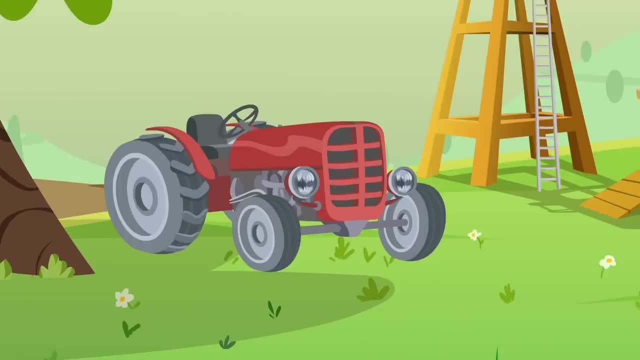 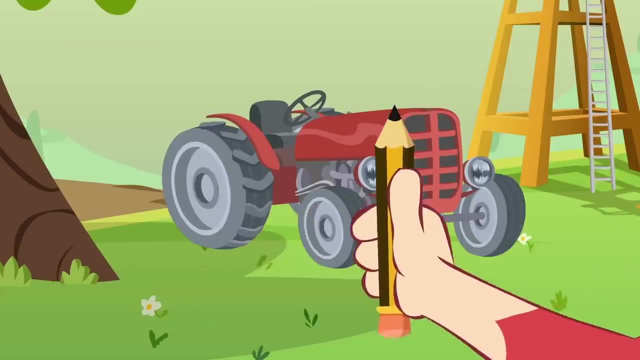 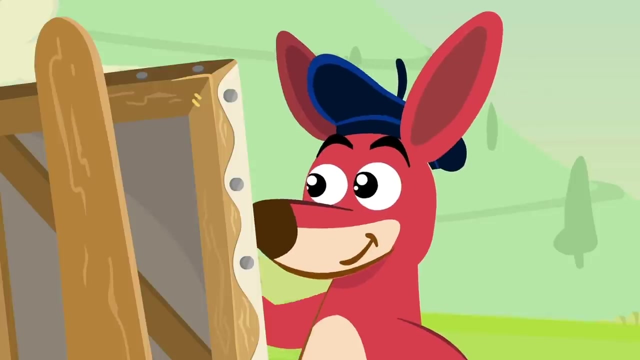 Today we're having a painting class with Kangoo. We're going to paint a beautiful rural landscape with a tractor. Let's measure it carefully And get to work. You're becoming quite the artist, Kangoo. Now it's time for the colors. 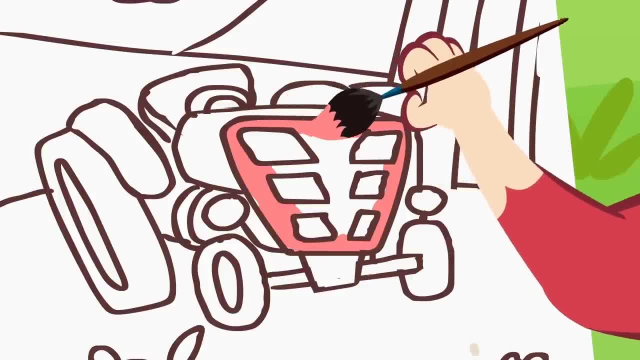 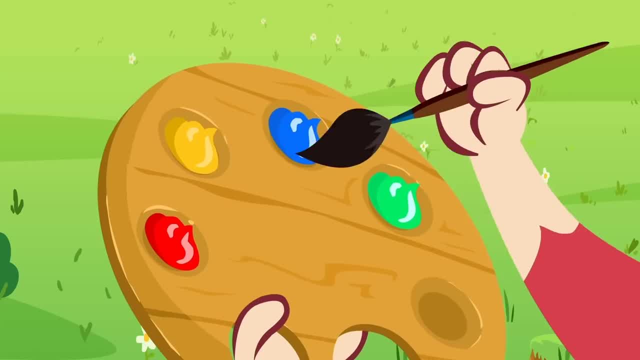 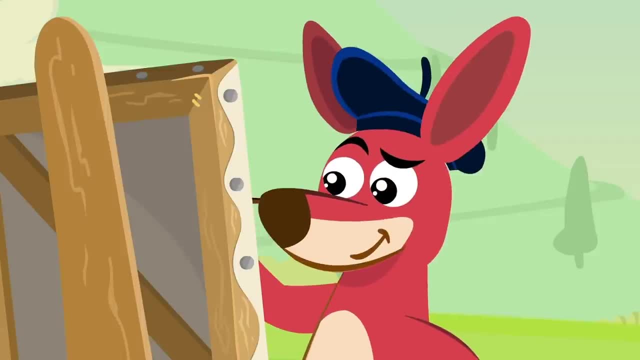 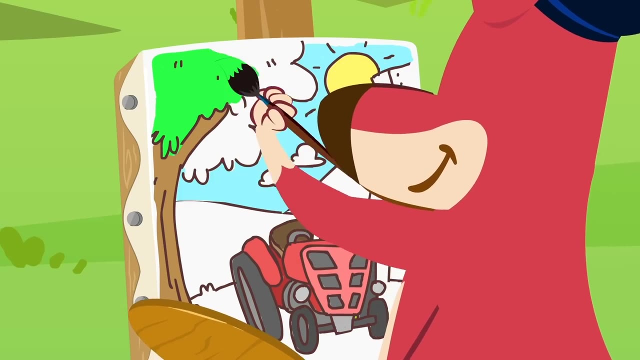 The red is for the tractor. What can we use yellow for? Exactly? for the sun, And the sky is a beautiful blue color. What can we paint with the green? That's it, the treetop. And one more thing is green. 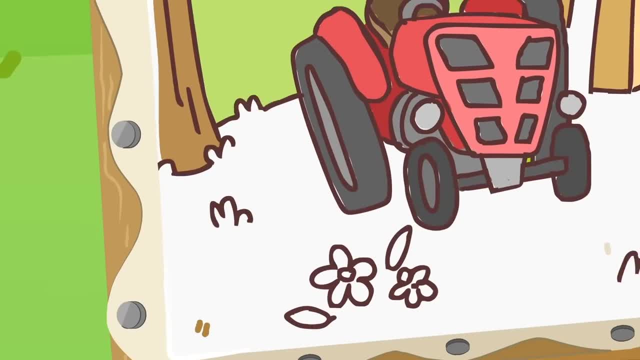 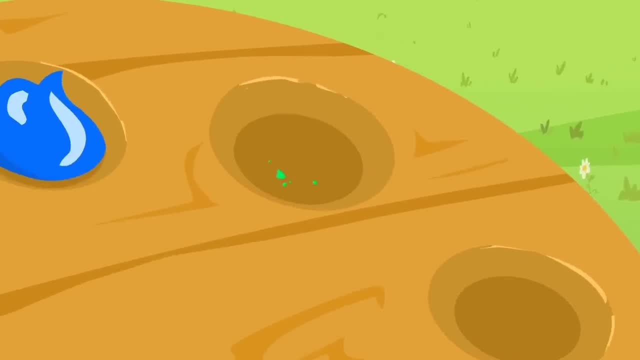 The grass. Uh-oh, we ran out of green. Hmm, let's think, What can we do? Aha, if you take a look at the tree, you'll see that it's green. Uh-oh, we're done with pictures.